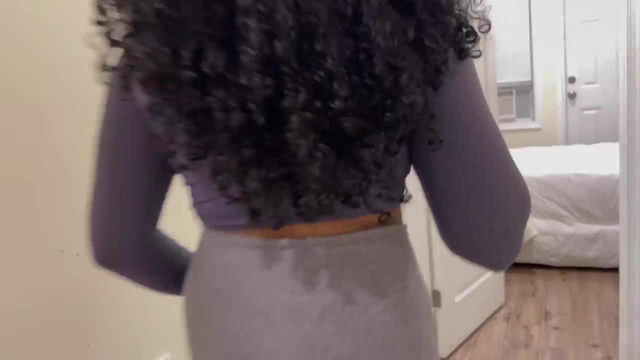 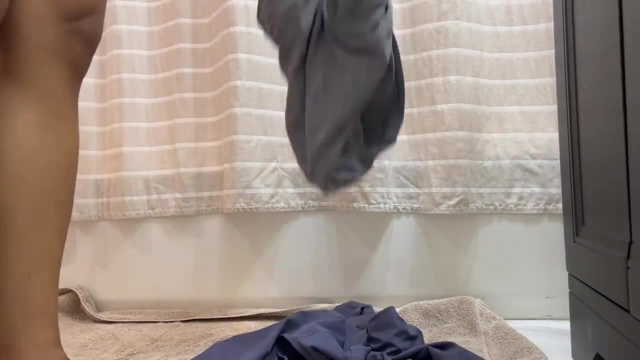 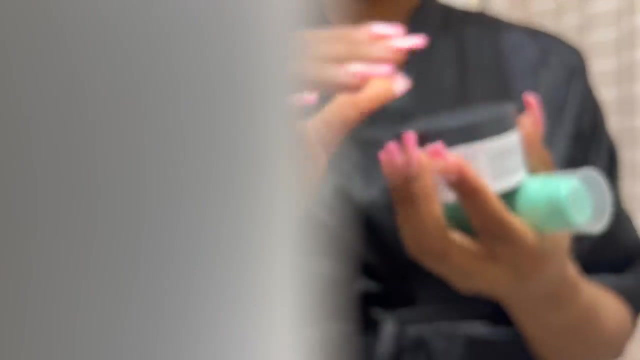 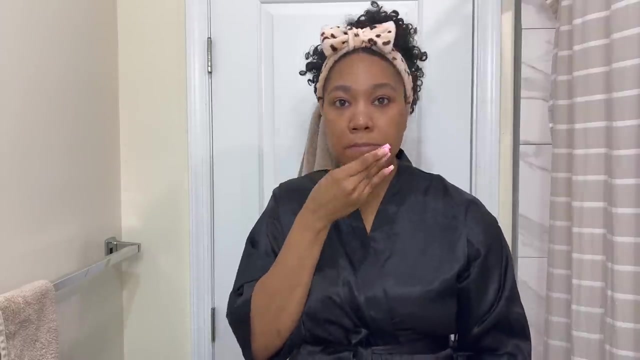 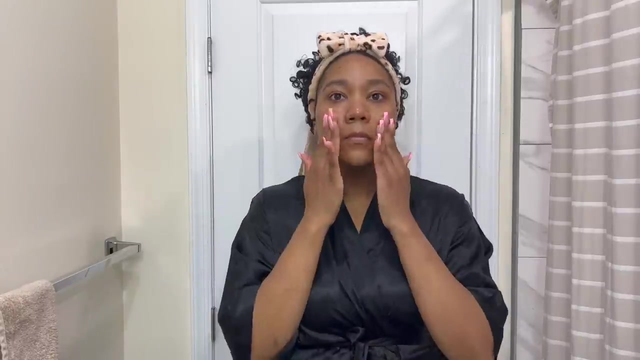 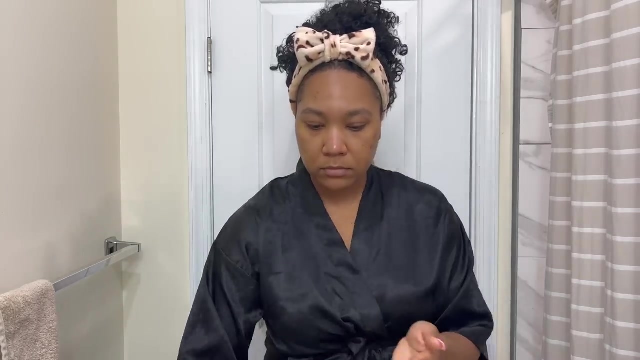 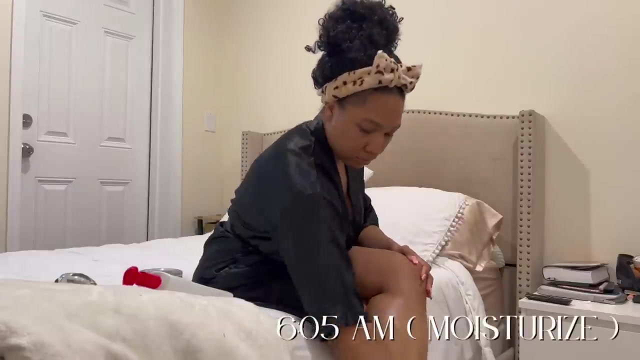 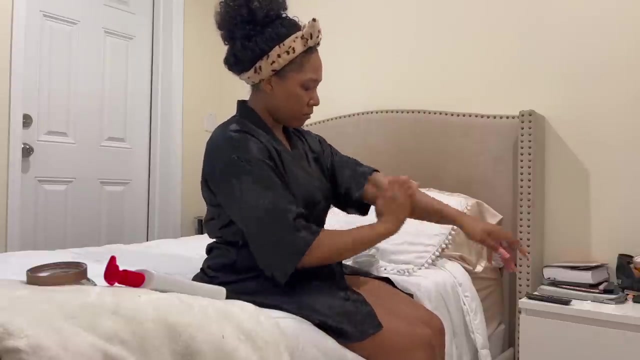 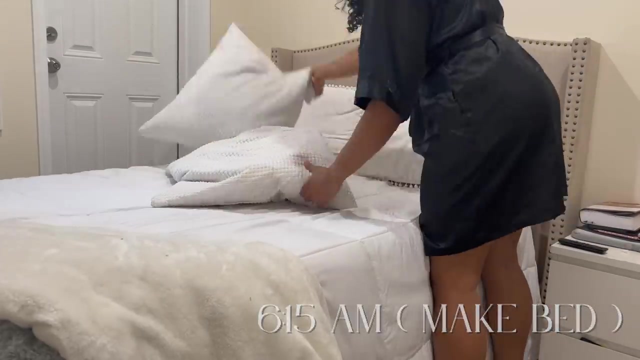 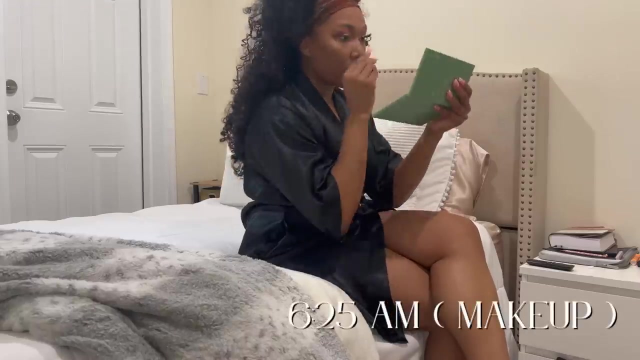 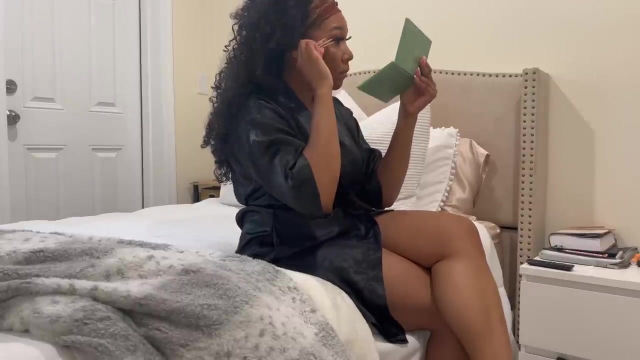 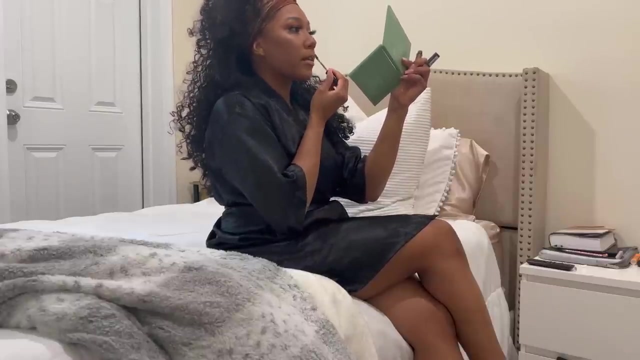 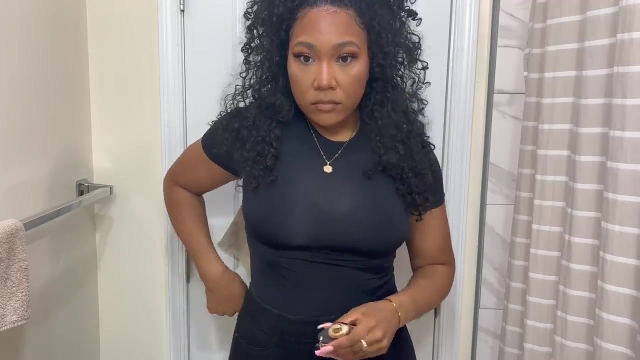 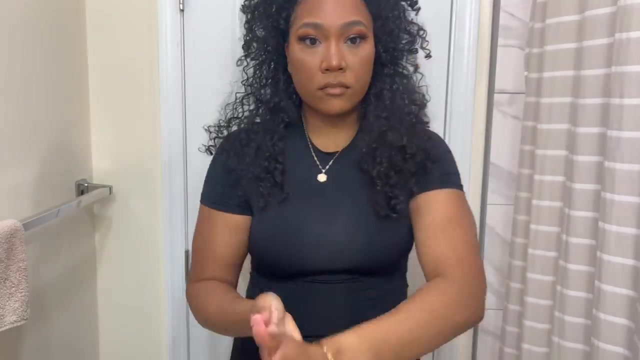 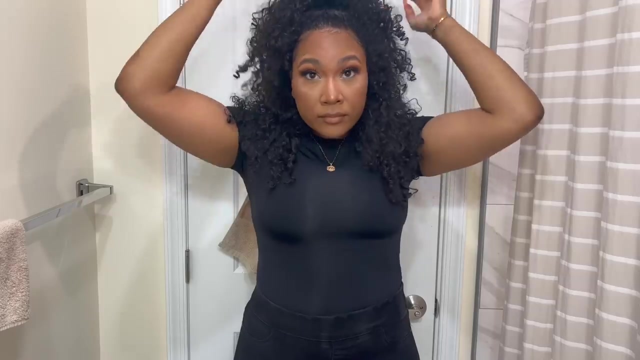 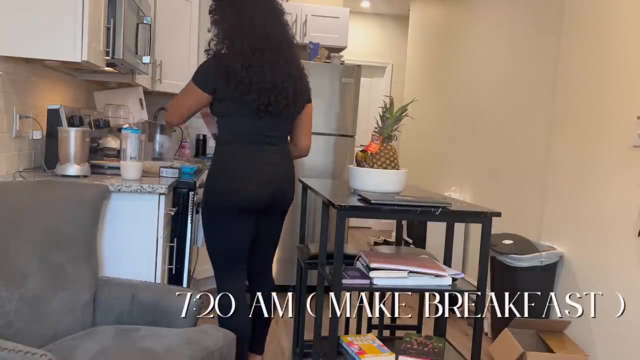 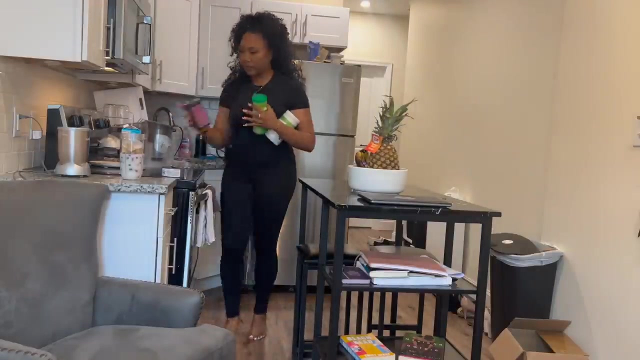 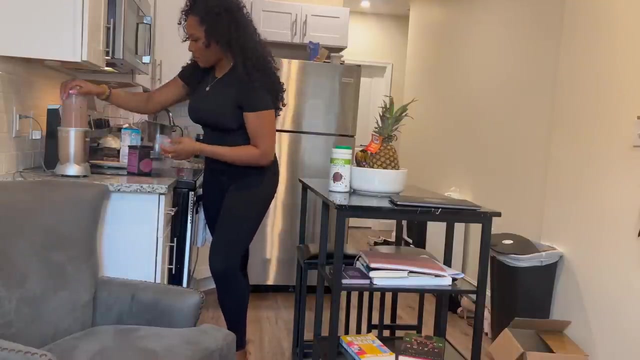 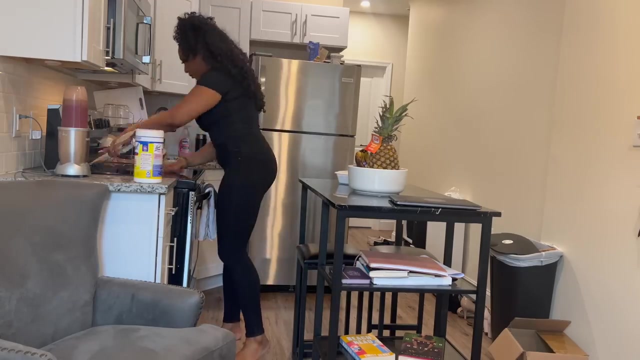 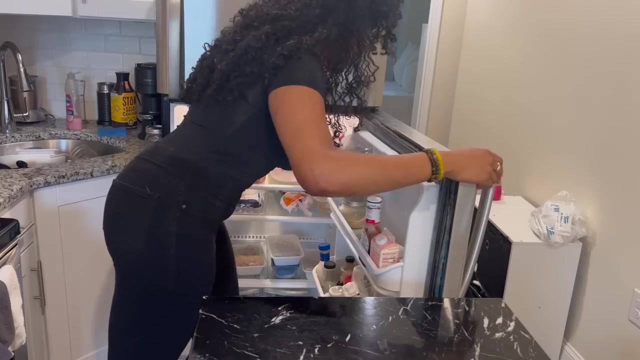 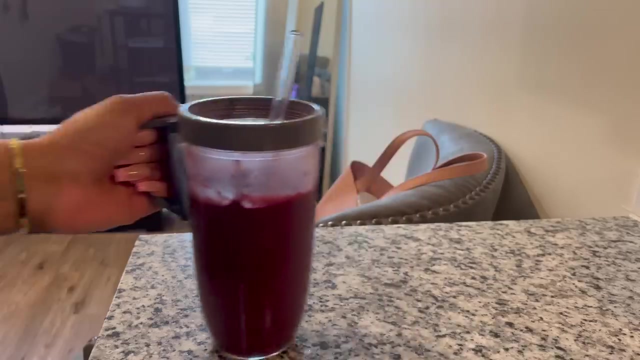 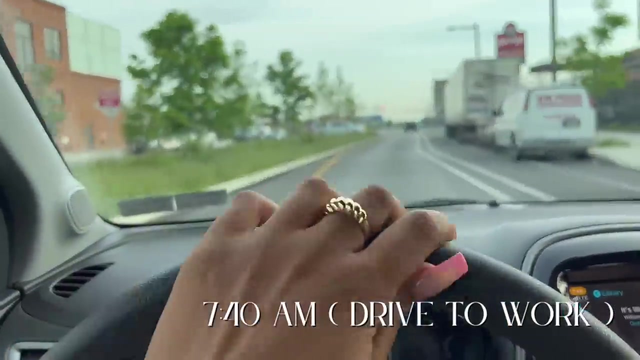 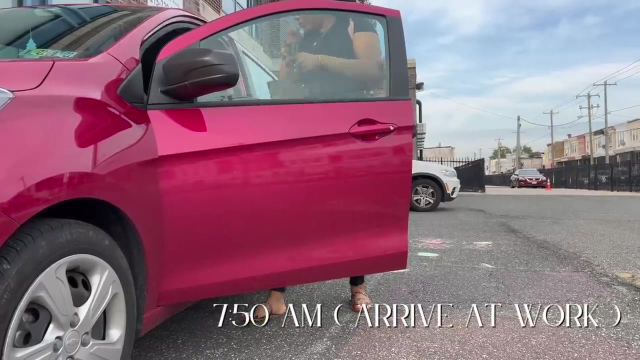 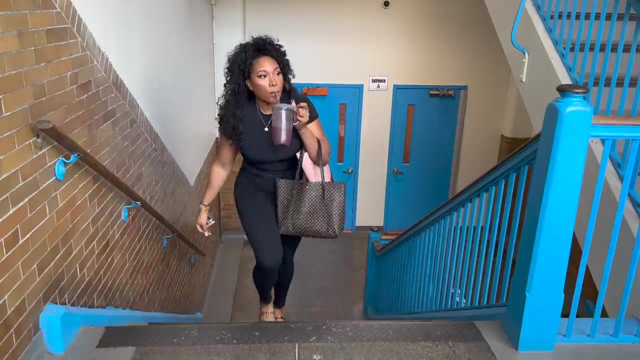 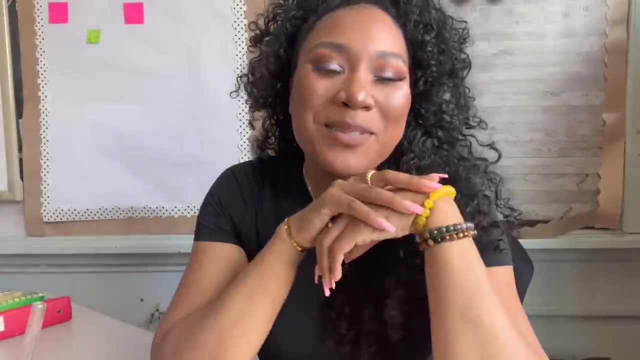 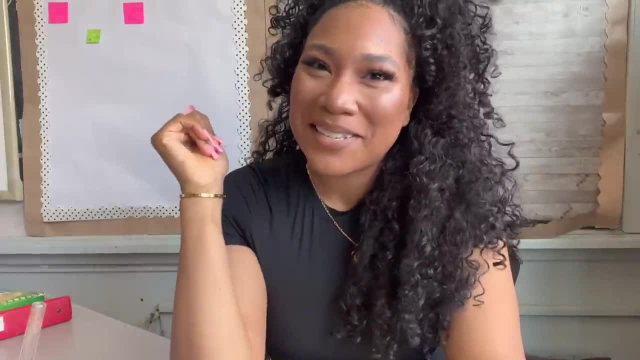 I'm so glad that you stumbled across my page. If you're returning. hey, Bessies, it's so good to see you again. So, as you can tell by checking out my channel today's title: we're getting into a day. 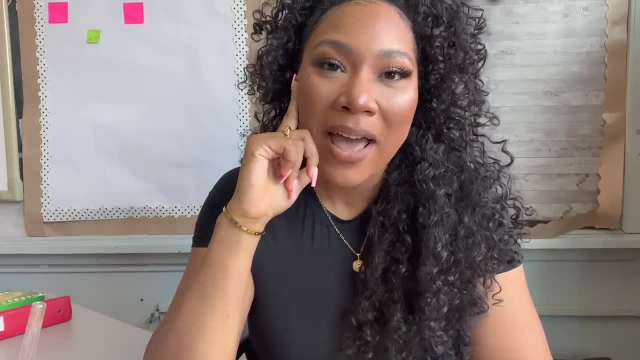 in the life of a middle school math teacher. I teach 8th grade math, So you've already kind of seen how my morning routine- the behind the scenes before I get into the building- goes. But now I'm finally in the building. 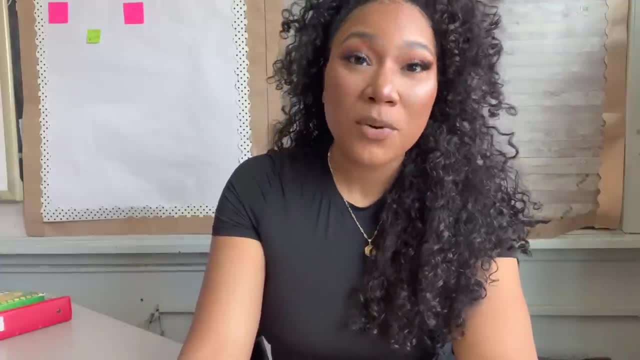 Basically, the plan is to take you through my entire day, So even when I leave the building, you can kind of get a grasp of what my day looks like. So I start every day at 3.45,, get to the gym by 4.30, which you've already seen. 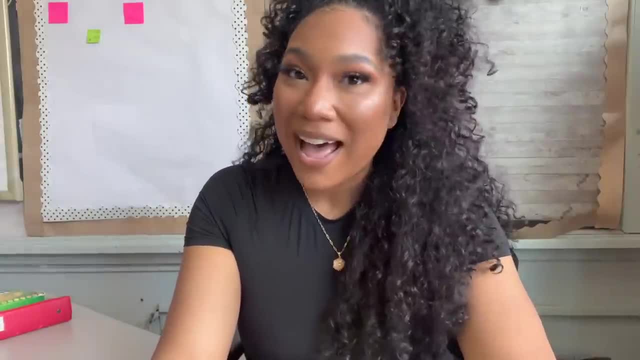 And basically my day just continues to go until I go to sleep. So it's about 8.15 and my kids get here at 8.45.. I got to the building around 7.50 today but I was like kind of. 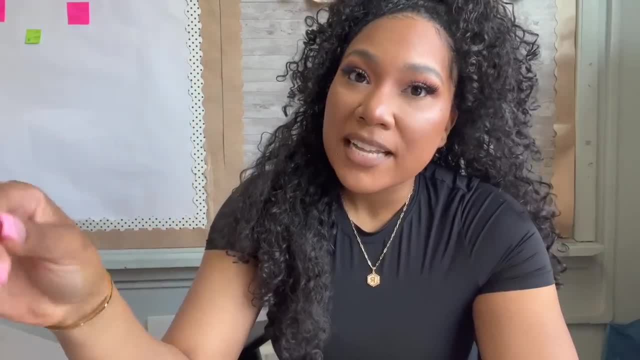 taking my time just like easing into my morning. So I need to take all the chairs down and sanitize all of the desks in my classroom. That's like the usual morning routine. Today is Friday, so the kids are working on a little bit. 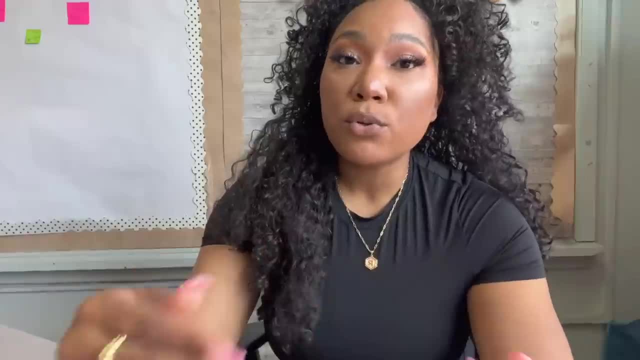 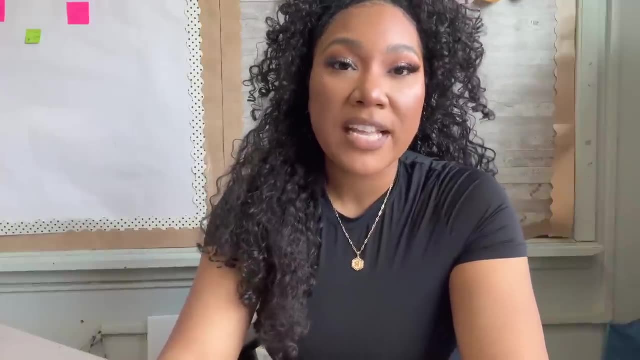 of a different schedule. So my students have a half day on Fridays. So usually Monday through Thursday I teach four classes but three sections. I teach for 90 minutes per class, except for my enrichment period, which I only have the kids for 30 minutes. But today 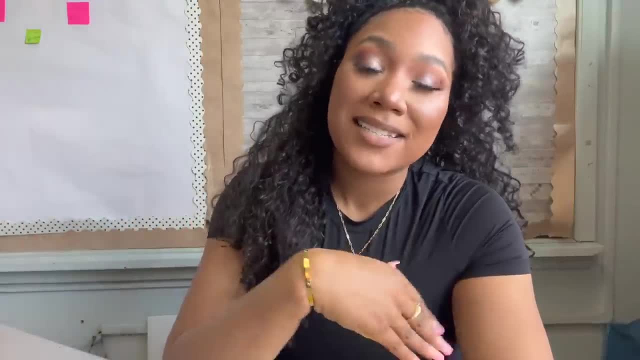 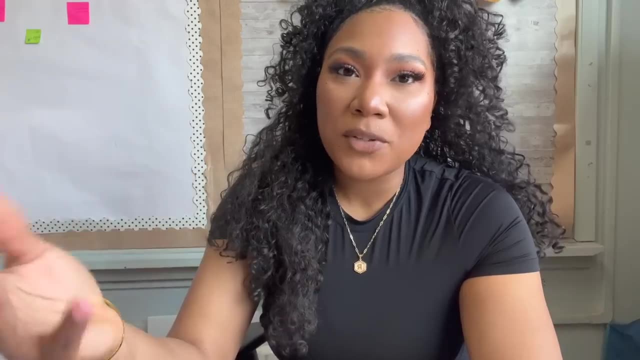 since they are operating on a half day schedule, I have all of my classes cut in half, So essentially I teach my first three classes back to back to back today. That's not the usual, but I'll probably do like a regular day. but 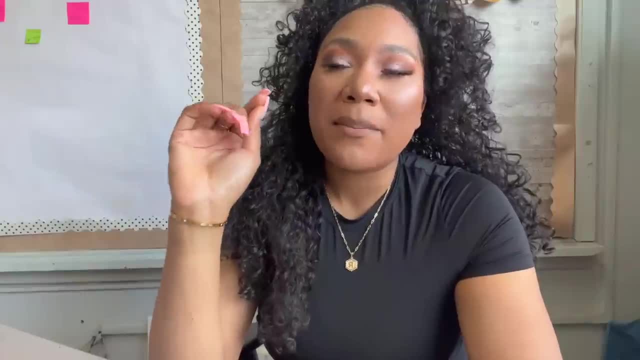 I don't know why I decided to pick up the camera and just do it today. It is what it is. So today I teach my first three classes back to back to back, So I have three classes for 45 minutes. Then the kids go down to lunch, which will give 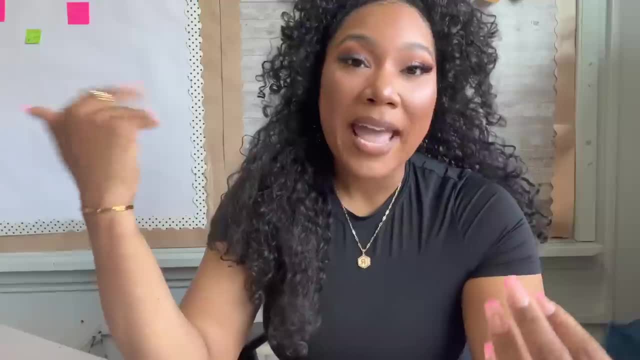 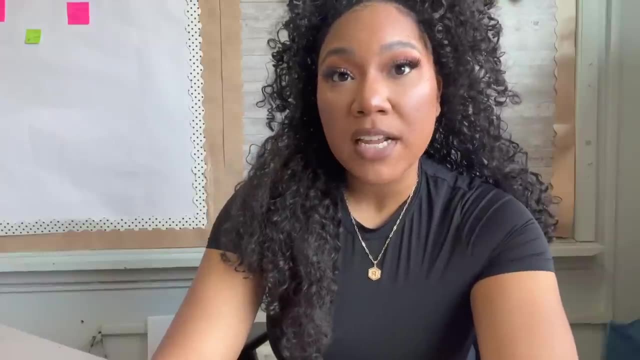 me time to have my lunch And then they go to their special or in my school's case, their expressive arts class. So they go down there and that's my prep period And then the kids come back up for caring school community, which is like a little like you know. 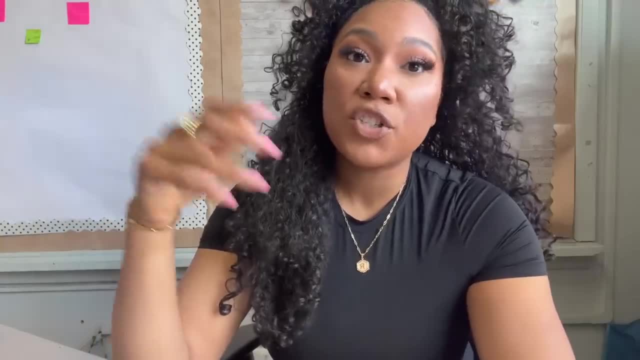 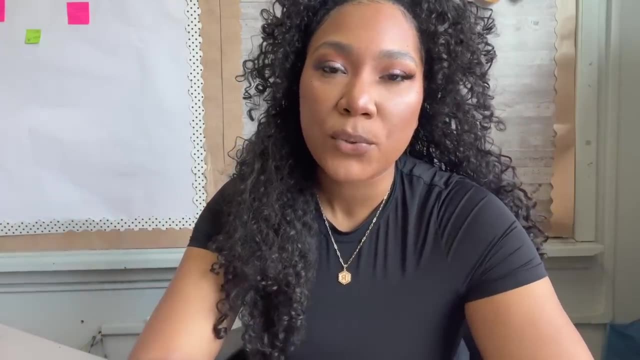 fun time, to have fun conversations or even like difficult conversations, just to like check in with the kids, see how they're doing, see what they have planned for the weekend, things like that. We always have some sort of like CSC activity that our school sends out as well, So we'll probably 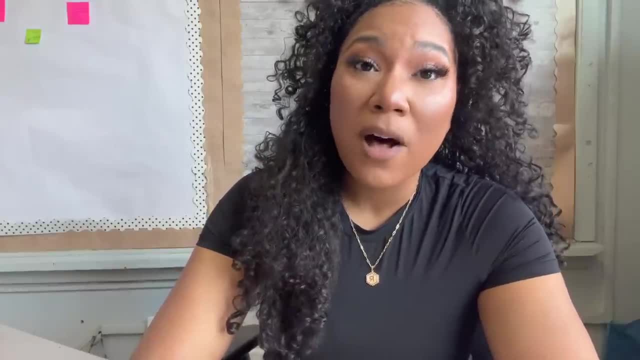 be doing that. But aside from that, that's what my day is going to be looking like while in the building, And then I don't know what after school is going to look like. but I know I have stuff to do, So I will just keep you posted. 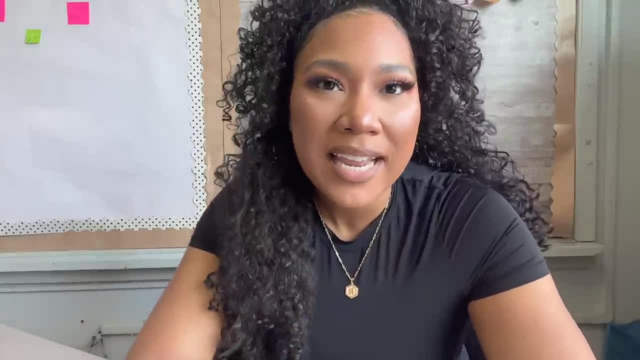 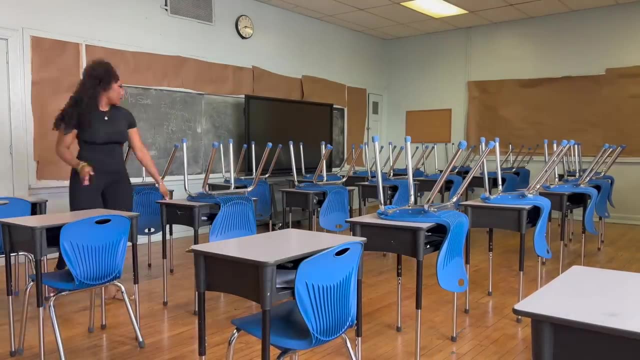 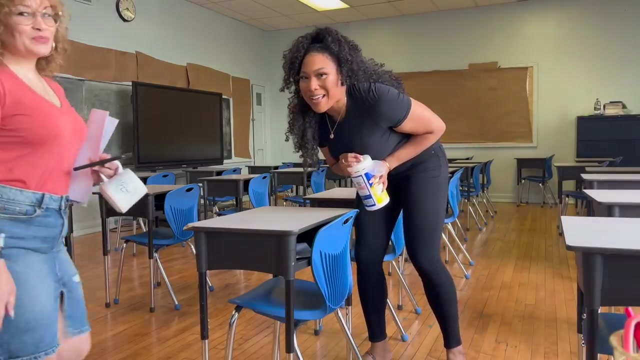 So I'm going to go ahead and start cleaning my classroom, just preparing before the kids get here. At least a little bit of that, and I'll talk to you guys soon. Music, Come say hi to my work, mom, Hi Laughter. 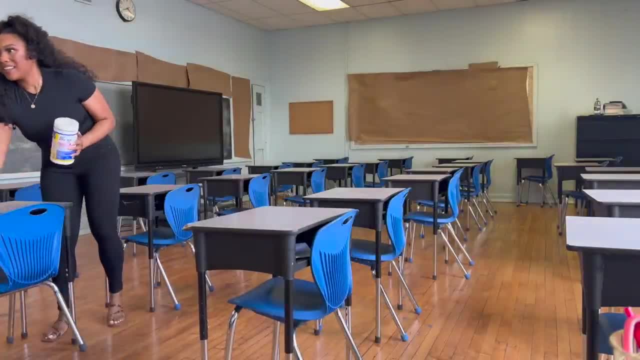 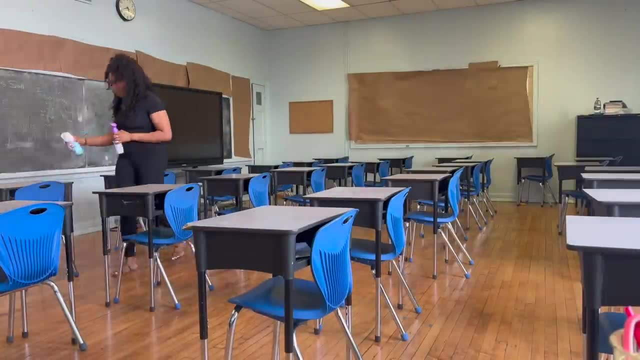 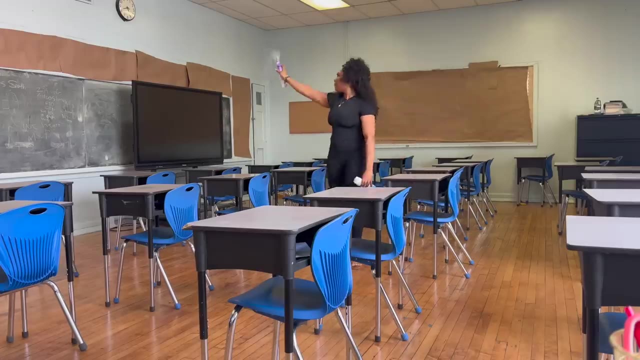 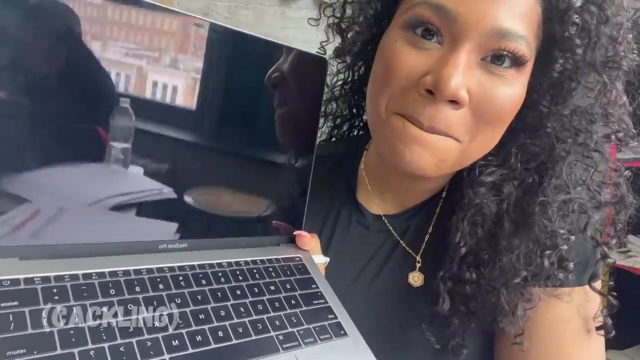 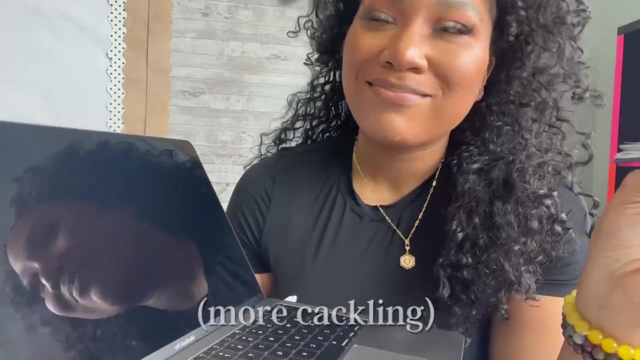 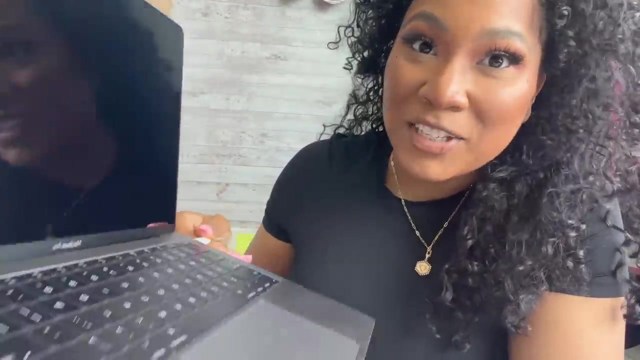 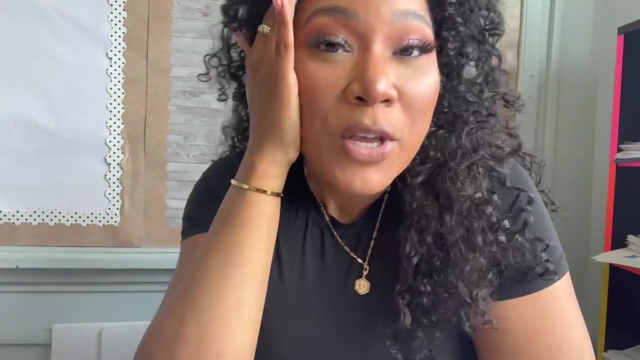 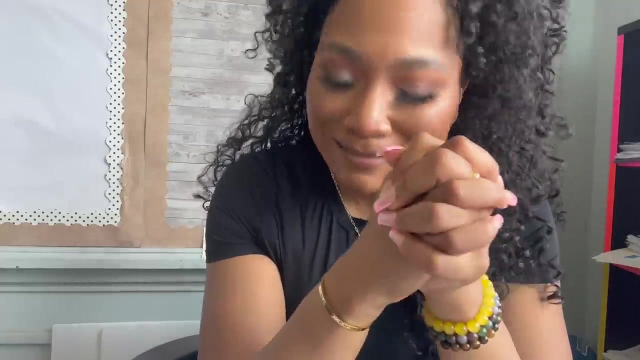 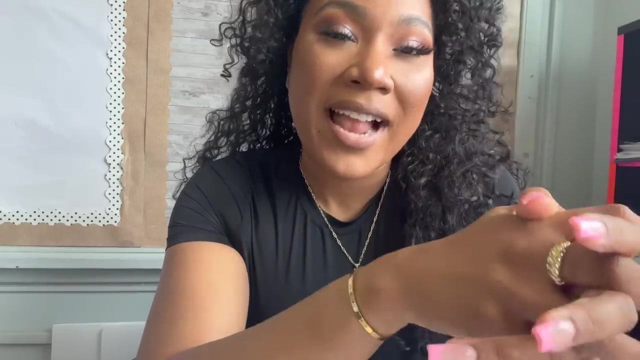 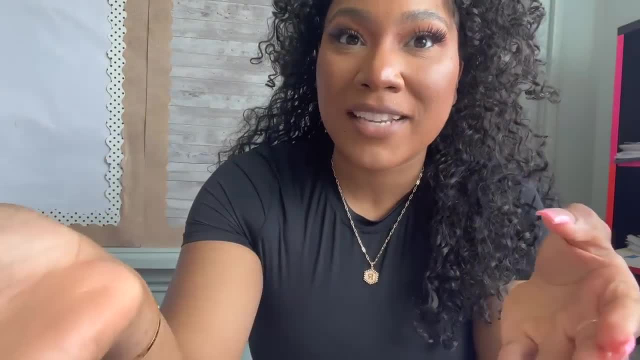 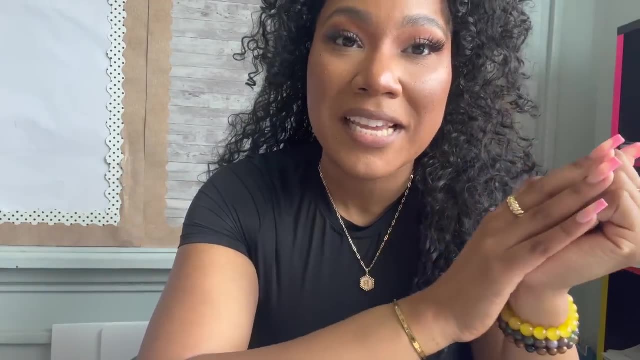 if I'm gonna be able to put it up or post it, because I don't know if I'm gonna have it access to it, like if I get a new computer. like I don't know if iMovie saves across, like Apple products, I don't know. so I'm trying to wait and see. so right now I'm in my first period, class first, and 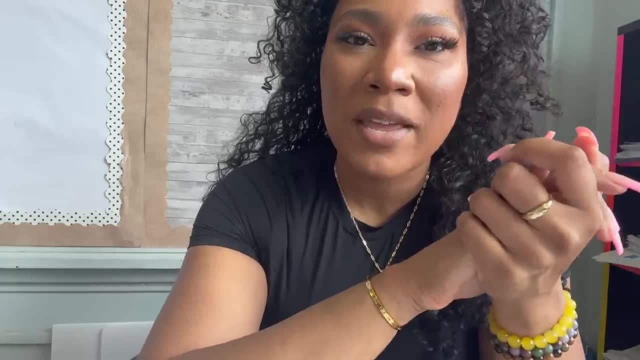 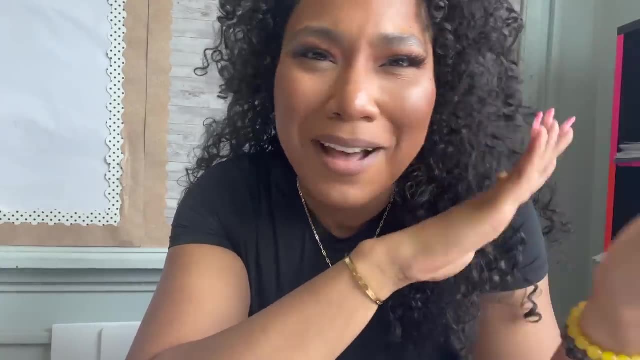 second period class. they are almost done. they're working on an asynchronous assignment so I can figure out what's going on. so I'm working on a student computer right now, but I'm a little stressed, so just I'll keep you posted. stay tuned, I'm vlogging. do you want to say anything to the? 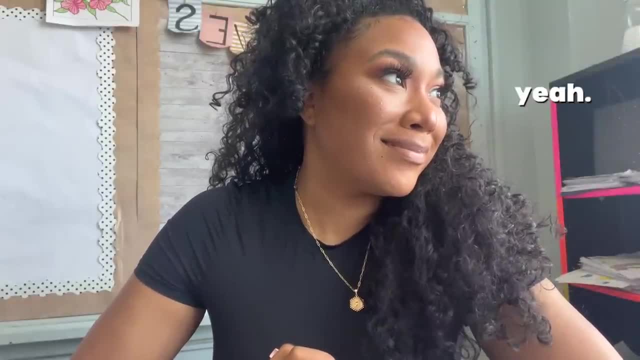 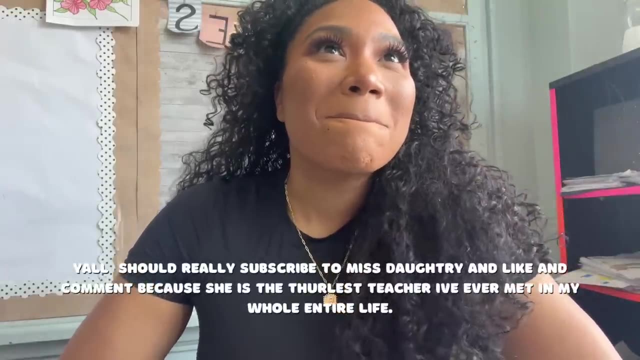 vlog. um yeah, subscribe to my favorite teacher. I would like to say something to the vlog. y'all should really subscribe to Ms Daughtry and like and comment, because she's the third teacher I've ever met in my whole entire life. your word, I appreciate your word to mother. 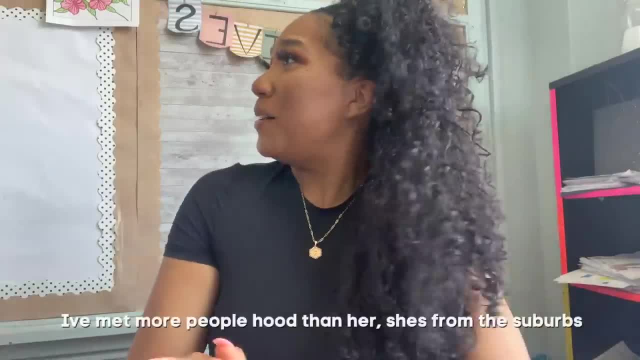 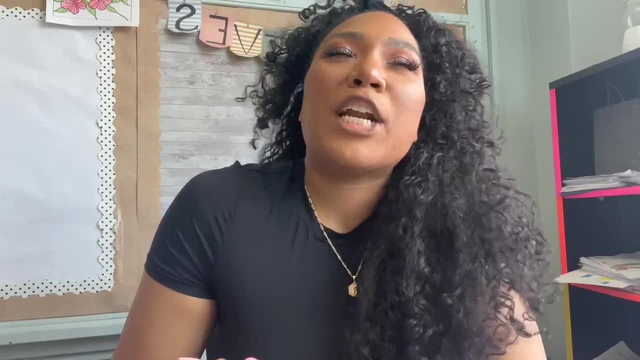 what I'm at. more people hooded her, she's from the suburbs- say no, you're a hater. I'm not a hater. it's giving a hater, it's giving. go get a computer and take a seat. hi, you are the best I'm selling. 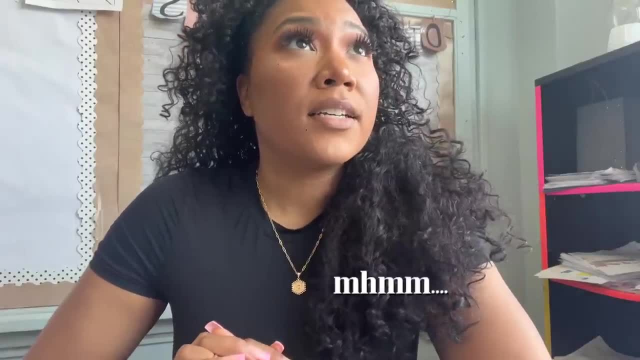 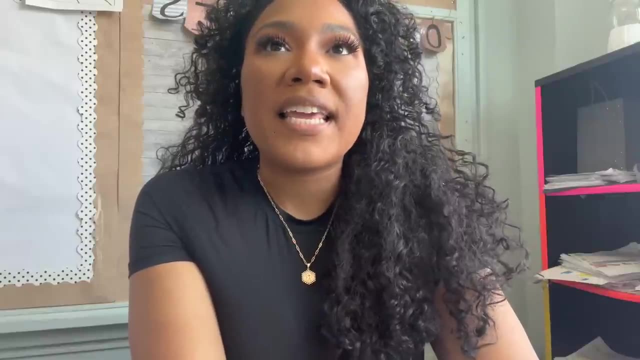 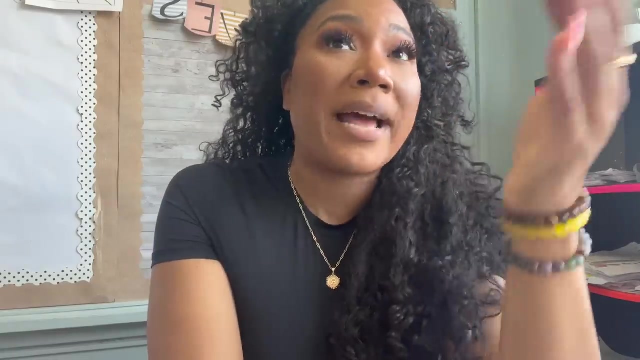 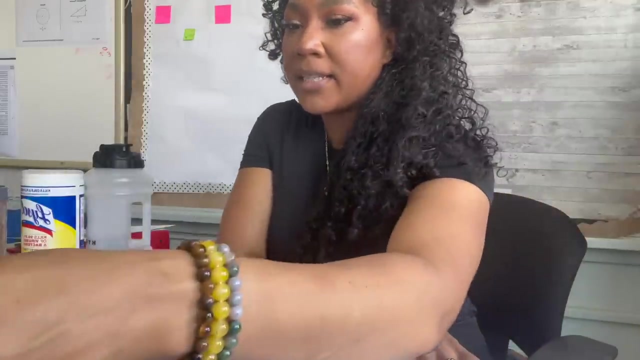 these shoes for 160.. you're selling your shoes for 160 dollars. somebody who got a team. oh okay, I'm not gonna repeat myself, so please listen up. you need to complete the assignment that I assigned on Wednesday. foreign. you get pierced your ears with this. all right, so it says the painting's completed. 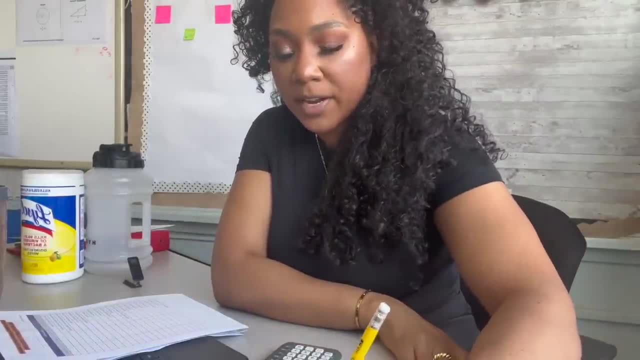 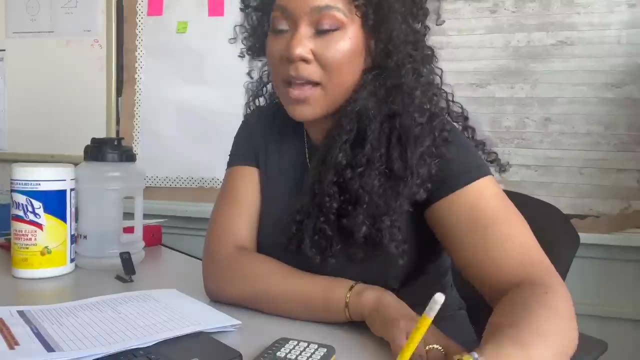 so there's ten, right? yeah, it tells me there's a 10.. so people's ten. so I'm gonna come over here and replace p with 10.. so I'm gonna get 10 over five. what's 10 divided by five? thank you, let's make that mixed number an improper fraction. you're going to multiply. 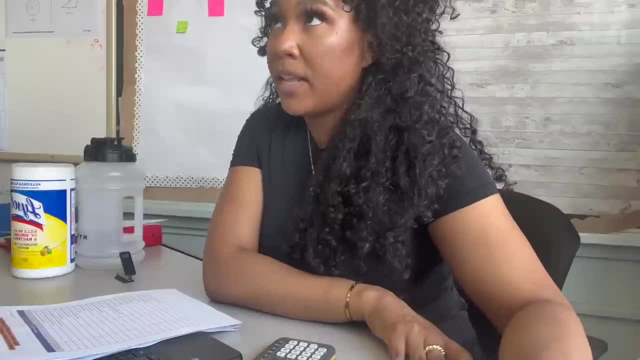 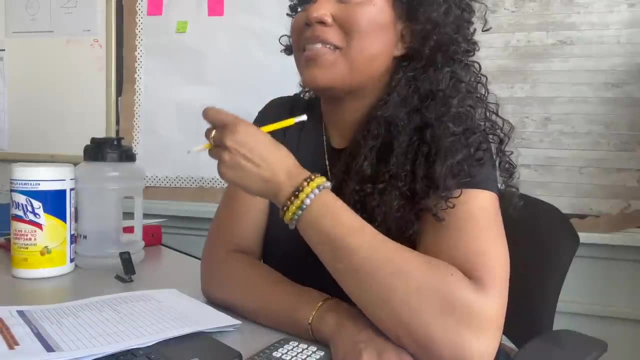 the denominator by the whole number. so five times one is what? and then you add the numerator, so five. Five plus three is what. So you have eight over five because you keep the denominator Reciprocal. Thank you, Teamwork makes the dream work. 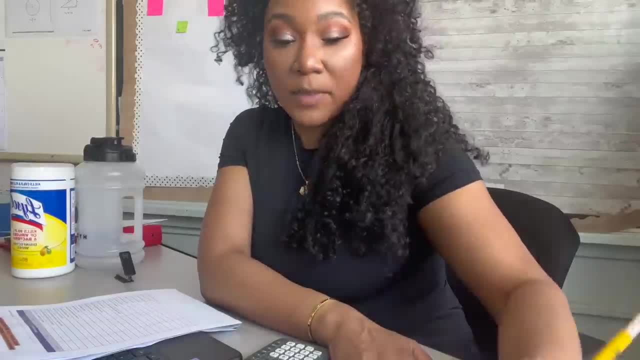 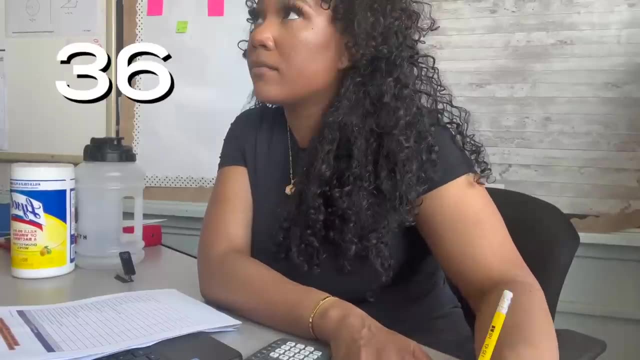 So I'm gonna multiply both sides by the reciprocal. So it's when I take the fraction and I flip it. So multiply both sides by five. over one D's are gonna cancel. It's gonna leave me with D equals what's eight times five. 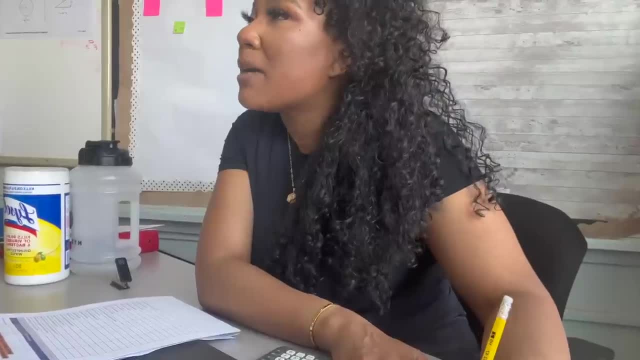 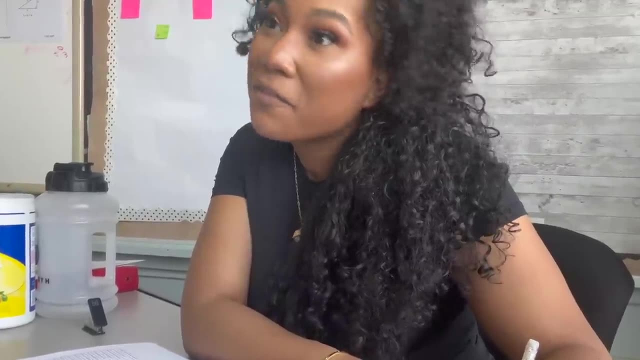 36.. You're- I mean maybe 48.. Eight times five, It's 0.. Oh my God, 45.. In what world is it 45?? You're fired, You're canceled. Eight times five, 40.. 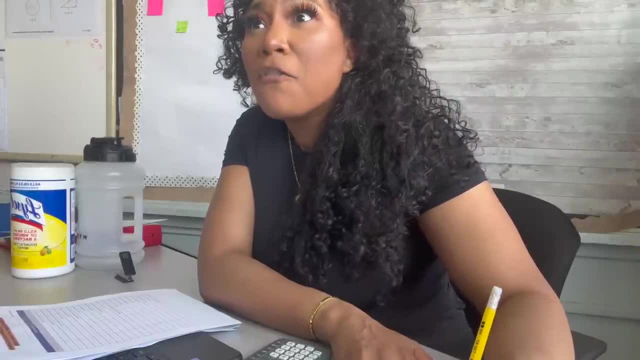 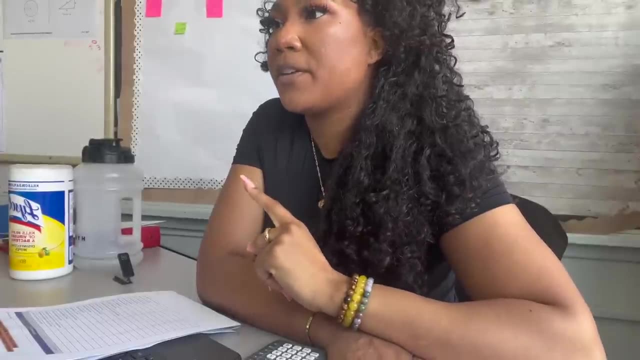 Who said 30?? It's yeah, it's definitely not. Don't listen to your parents. It's 40.. Who else needs help? Well, Chance was up here first. I just- Chance was up here first. Well, he's not here anymore. 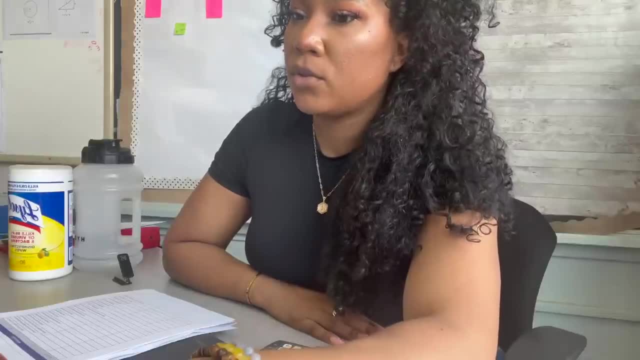 He's right there. Yes, he is. Go back to your seat, I'll be right back. What's the hypotenuse Can you show me on the triangle? What's the hypotenuse of the triangle? Sorry, Oh wait. 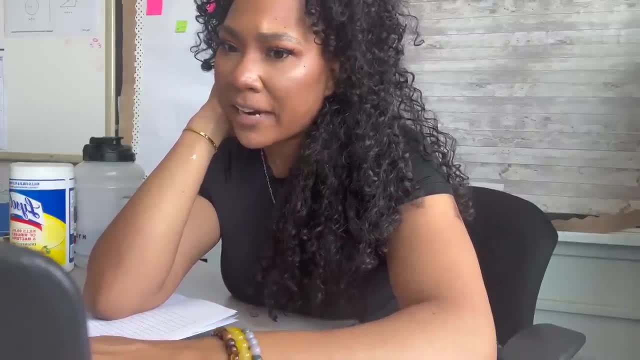 Why is that wrong? Why am I wrong? Oh wait, no, I'm right. right, Zero comma four. Yeah, Okay, So a vertex is done. Okay, All right, You know, Ms Dr Ra, check yourself. 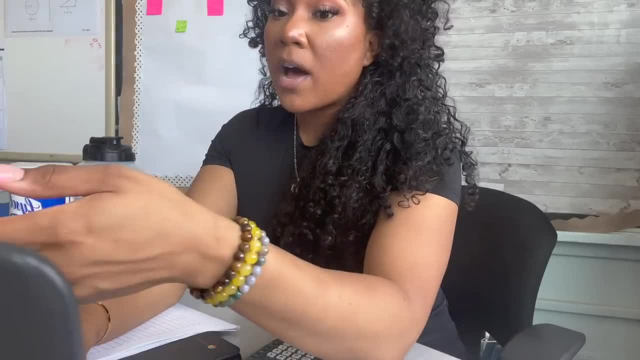 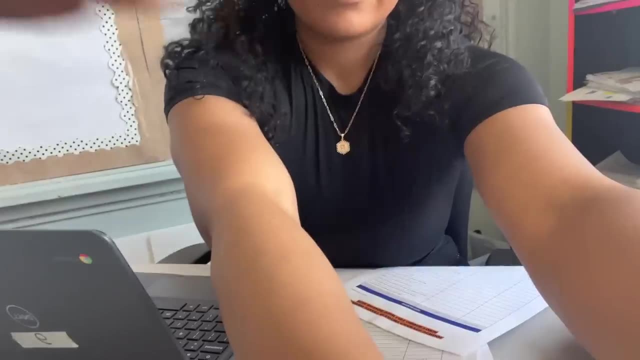 Does the slope of a line ever change? No, That's why it doesn't matter what two points I pick on the graph and do my rise over run. It's all going to equal the same thing. Nice job, All right. Look, it's like a little rhino. 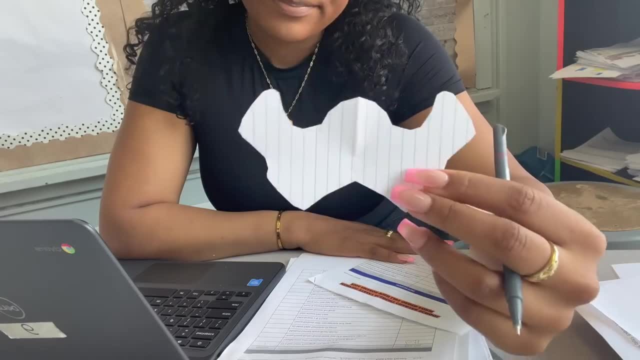 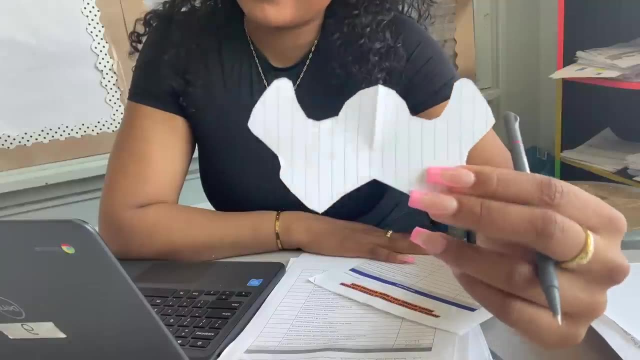 I mean a little rhino man. A little rhino man. Yeah, he's like a bad guy with two horns and then a hat, Like one of them. viking people. A viking- Oh, That does make sense. Do you want me to keep it forever? 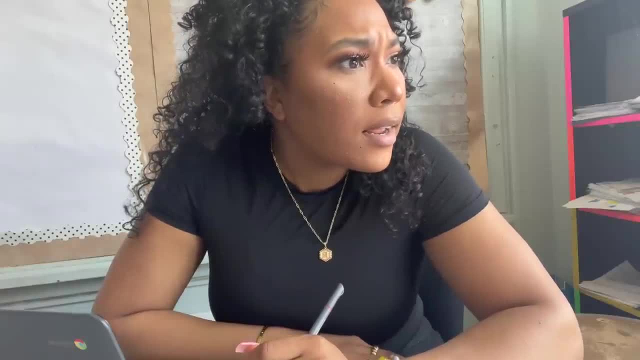 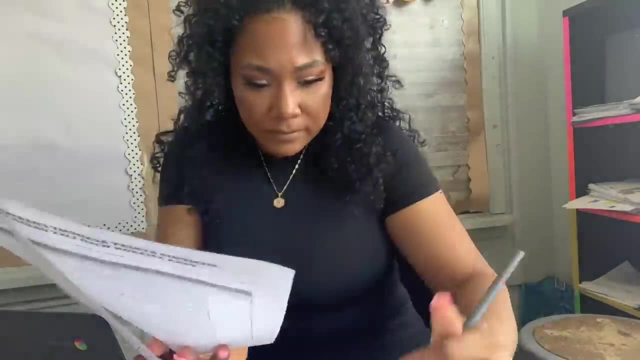 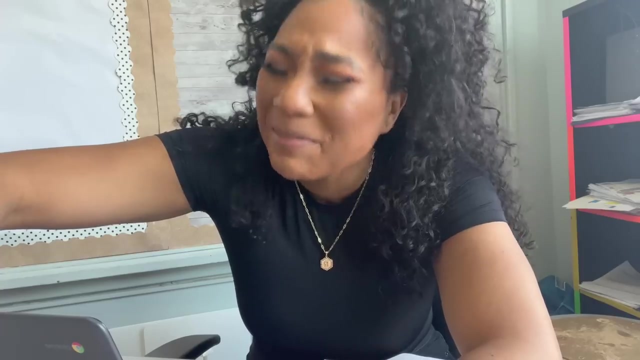 All right. Why are you on the floor? Why are you on the floor? Okay, Well, if it makes sense to you, then you go with it. See, this is why. Yo, oh my God, It was how you said it. 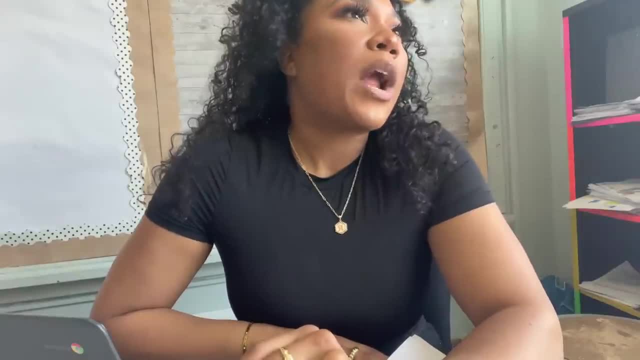 It was wrong. Oh my God, It's okay. It's good that you are able to reason through, though, Like I like to, I like to hear that you are actually thinking about it, You know? Okay, Hi Noodle. 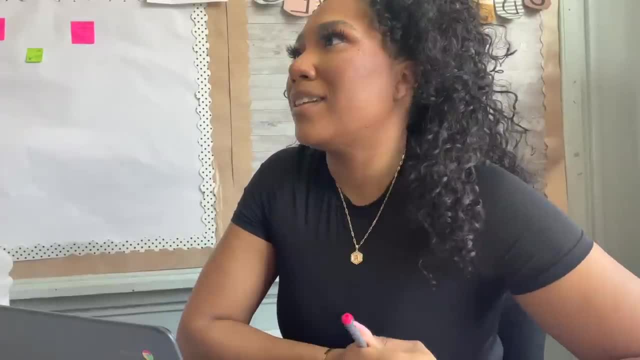 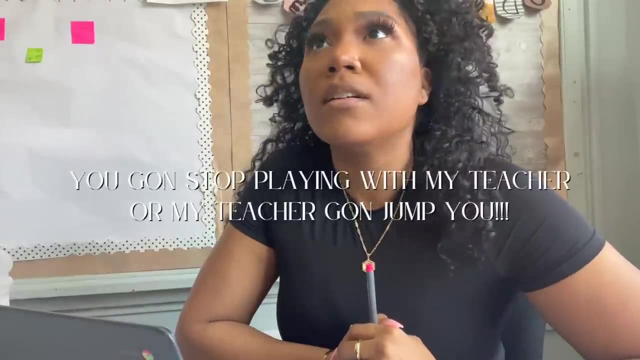 How's your plan going? It's going. How are you Good, Hey Daughtry, Hi Izzy girl. No, people want to be like that. Your niggas pee on your niggas, Ah Yeah. 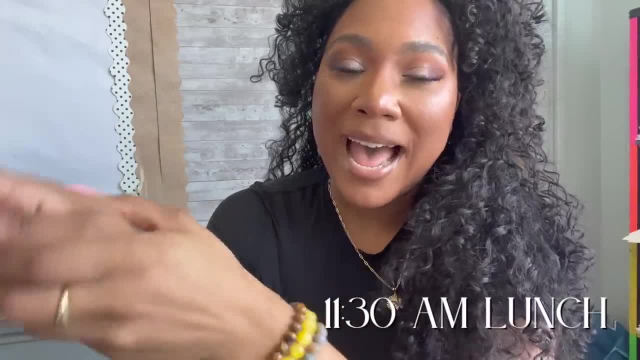 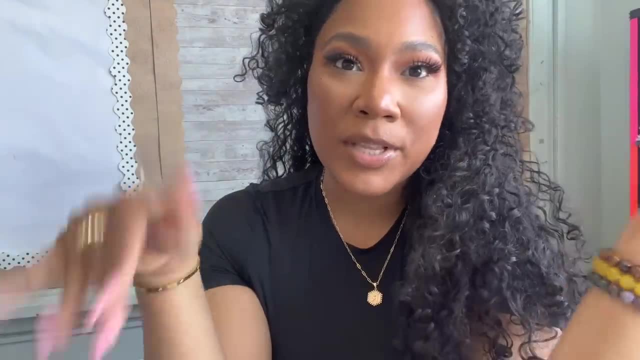 Yeah, So it is currently my lunch time And I have a couple of kids that want to come up for lunch. I'm going to vlog really quickly and update you guys before they get up here. So basically, during this time, I usually don't allow kids to come up. 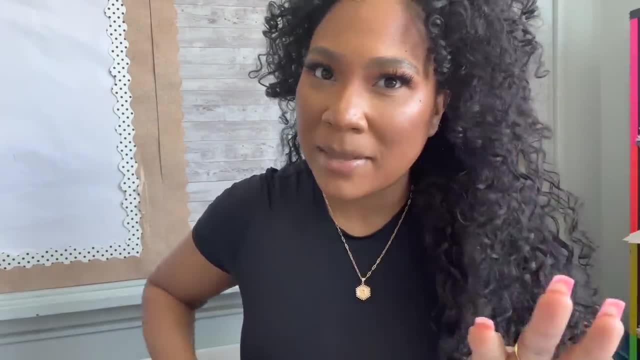 I'm up on Fridays, but they can come up today because the end of the school year And you know I'm just letting them be great. So I usually let the kids come up, like Tuesday through Thursday, not Fridays. But I'm letting them because like it's fine. 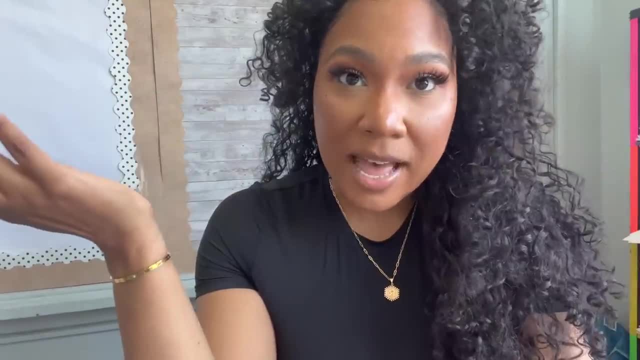 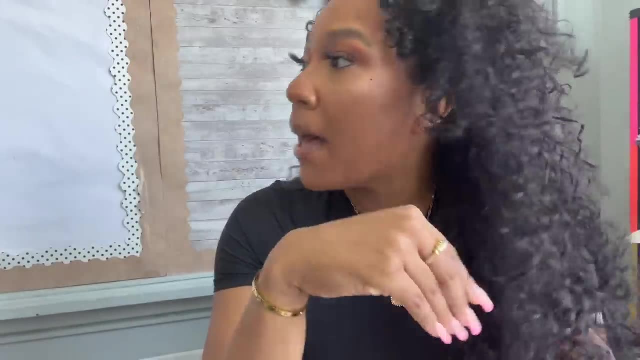 I don't really have much to do, So I like to use this time to obviously have lunch, And then I also need to just like straighten up my desks and re sanitize the desks, because the kids have sat in them all day And I have one more class today coming up. 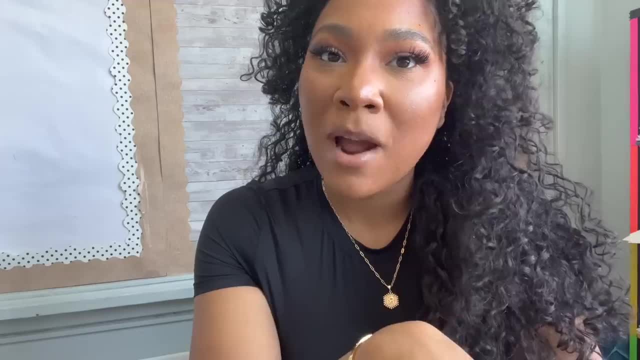 I'm going to go ahead and just organize my class: let the kids have lunch, probably try to eat my lunch if I don't get it, And during my lunchtime I do have my prep period right after, which is like a nice 30 minute break. 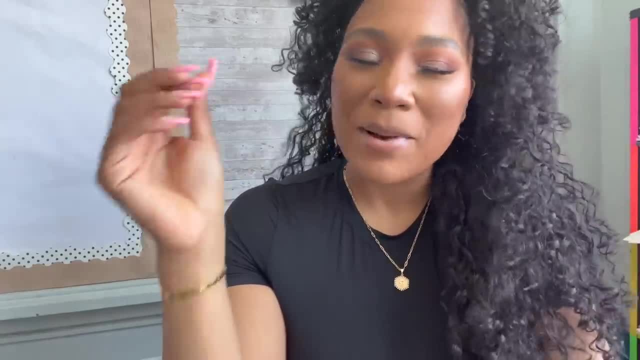 with the kids back. So this is basically what it is. Teachers don't really get much of a break, And even on their breaks they're still working. So just keep that in mind. But I will talk to you guys in a little bit. 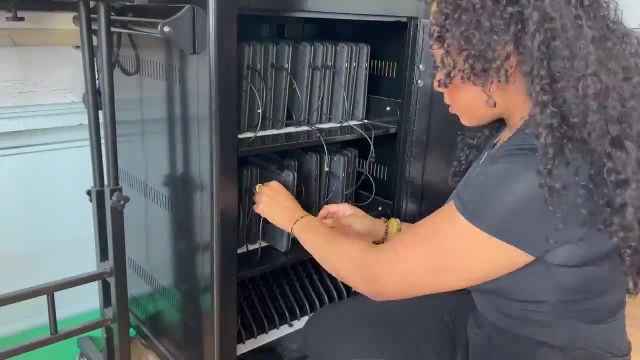 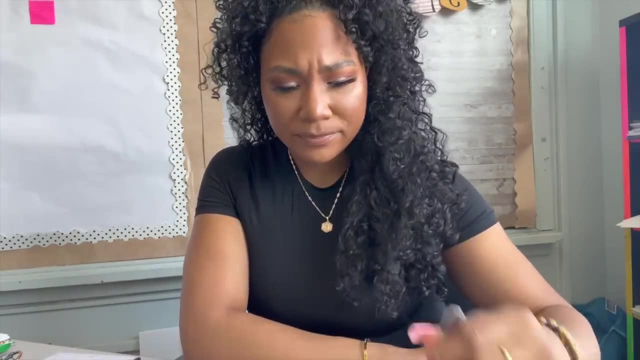 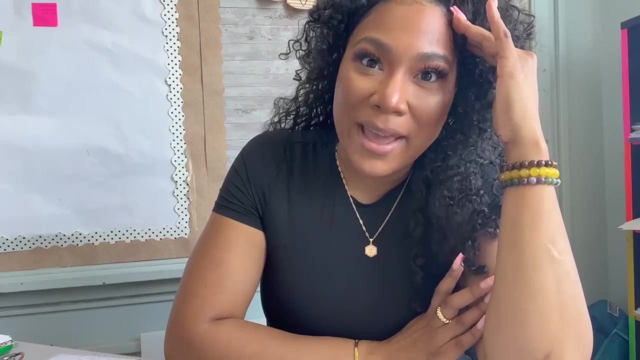 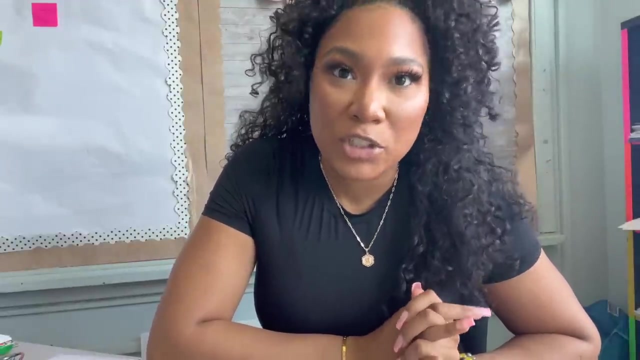 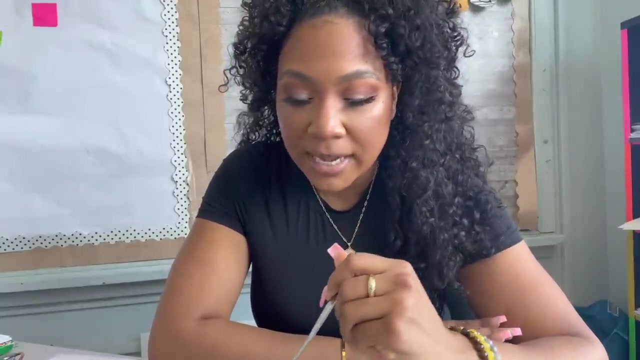 i shall k q. Okay, so today has been a little bit unpredictable, seeing how my computer basically just like crashed. The screen is black, Nothing is happening and I'm stressed out. So I gave it to the IT department downstairs. well, there's no it guy in today, but i gave it to the woman who like deals. 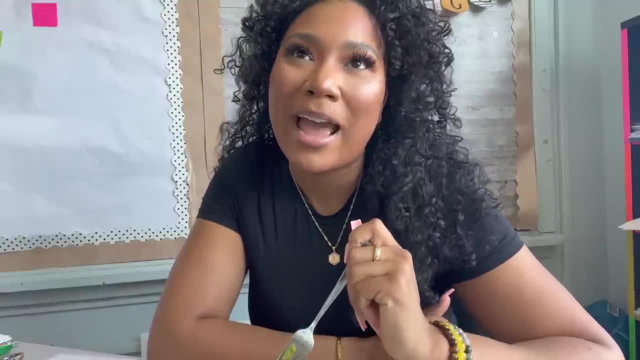 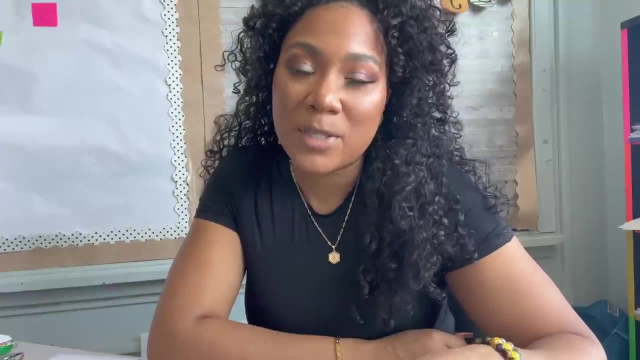 with that stuff and i scheduled an appointment at the apple store today at 4: 45 to get a new mac, and this one will just be for me, because i can't go through this again. i'm a little bit stressed because i was supposed to get three videos up this week and now i'm only going to be able to. 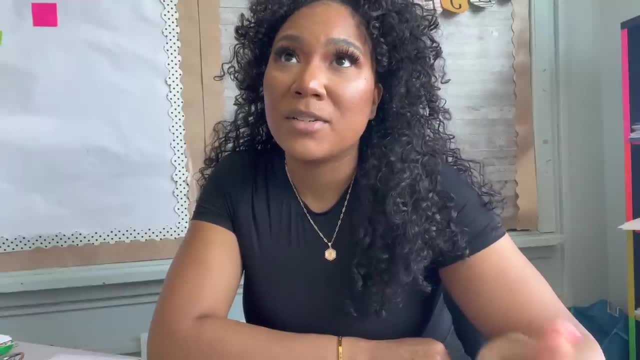 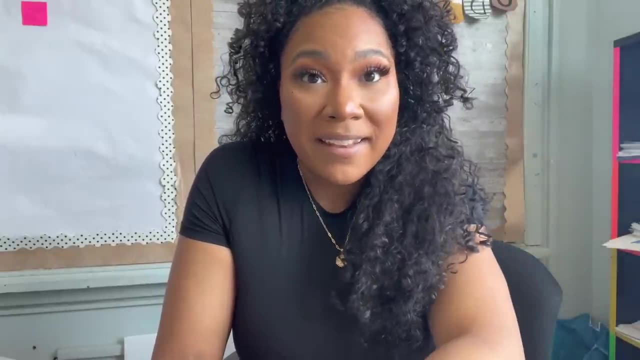 get two. hopefully i'm able to get the computer today too, like i. i just i'm really stressed out. hold on, sorry about that. i had to go get some students from the cafeteria because they were not notified that their gym teacher was not in today and that they needed to come back to the 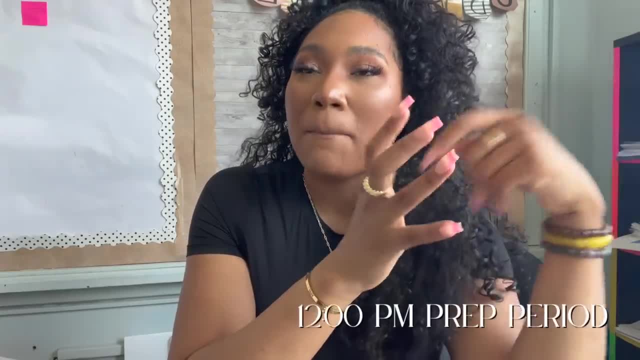 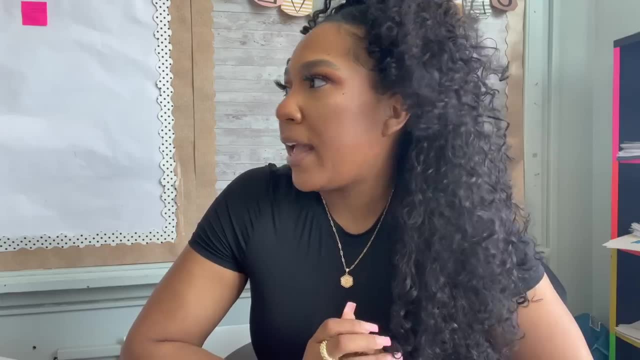 third floor. so basically now it's my prep period, but i'm going to enjoy the rest of my lunch, because i didn't really get a chance to eat my lunch. i'm also going to straighten up a little bit too. i already like wiped down my table, and i also need to grade a couple of assignments now. usually i 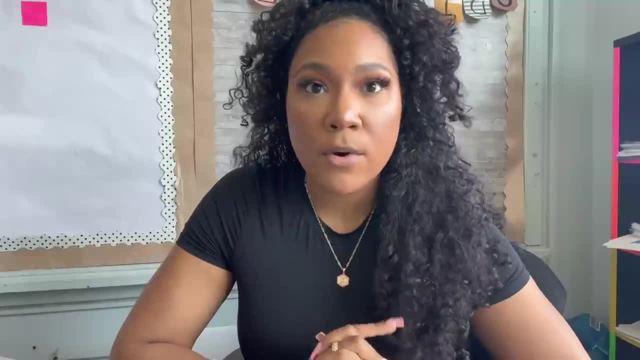 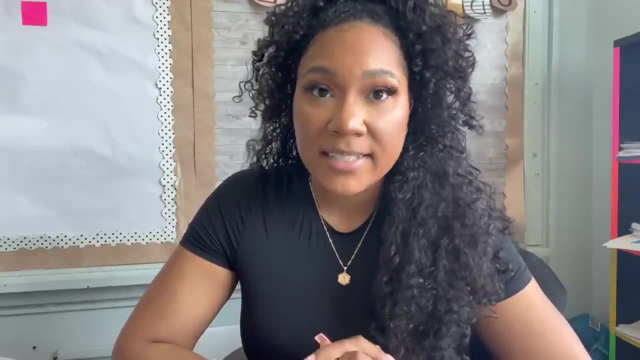 would take this time to email parents, make phone calls home, just other professional responsibilities. but because my computer situation right now, i'm not sure if it's going to give me access to my work email on the kids computer. i'm going to try it. if not, i'll just send them from my phone. 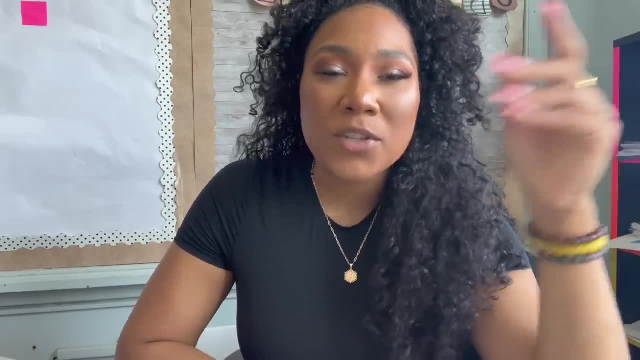 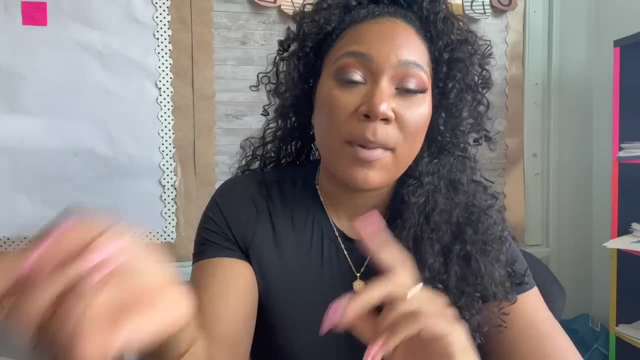 um, which is no biggie. i also sent a ton of emails this week. so basically, what i like to do, just to not overwhelm myself, is that i teach four classes but three sections, so i get one of those sections back for another class for an enrichment period, and what i do is i designated a day of the week. 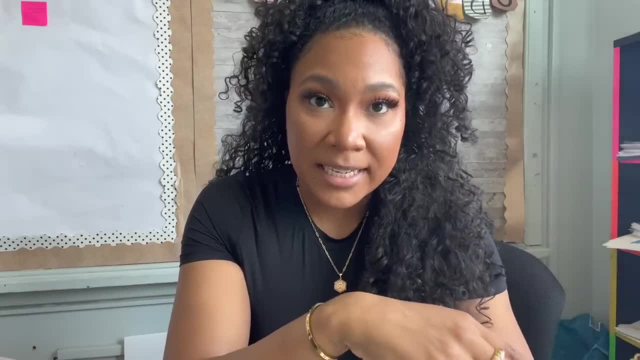 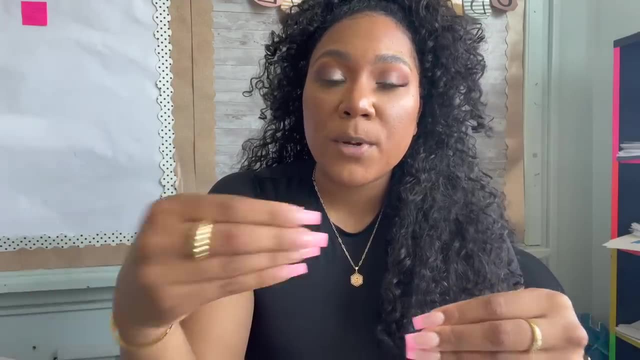 to focus on those specific kids and then contact the parents as needed. so, like i teach sections eight four, eight five and eight six, so on mondays if i need to send home updates or emails about specific students regarding behaviors or grades, things like that, i send the parents the 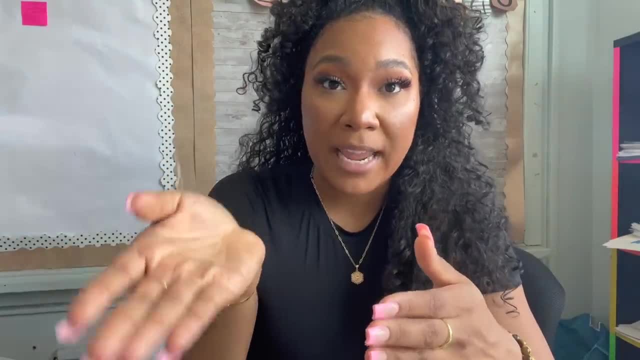 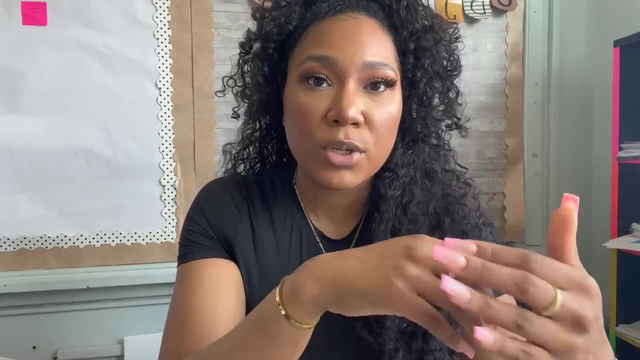 emails on mondays for that specific section, then tuesday i move on to eight five, and then wednesday i move on to eight six. so usually i don't really have that many emails to send on fridays, because i usually try to get that done during the week. because one thing about me is that i don't want. 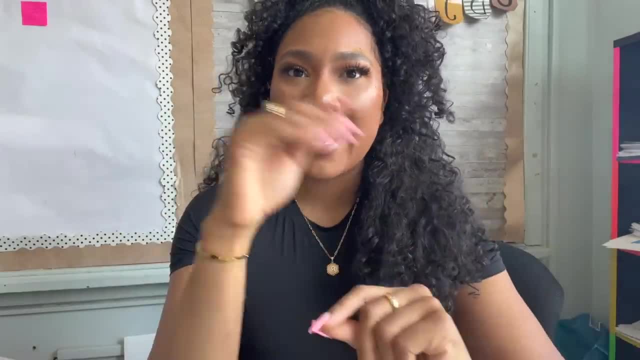 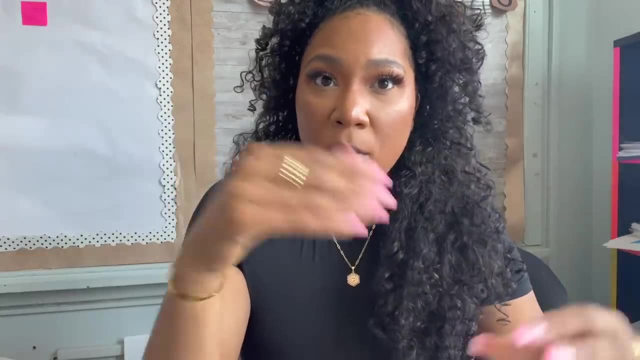 to take my work home over the weekend. it would be kind of a lot to have to be grading and bringing home all my work stuff on the weekends. i don't like to do that. just kind of reduce the likelihood that i'm gonna get teacher burnout or i'm gonna. i'm gonna. 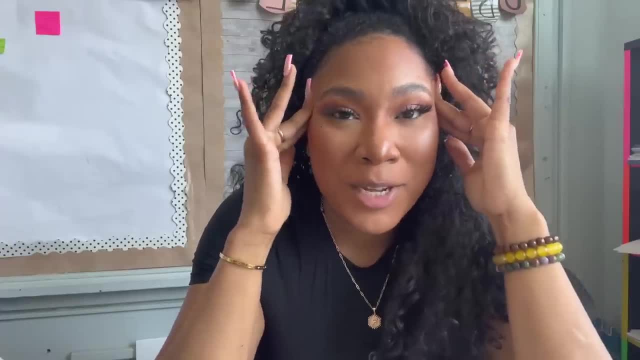 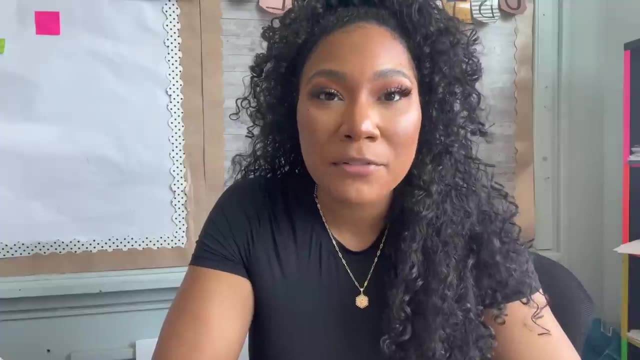 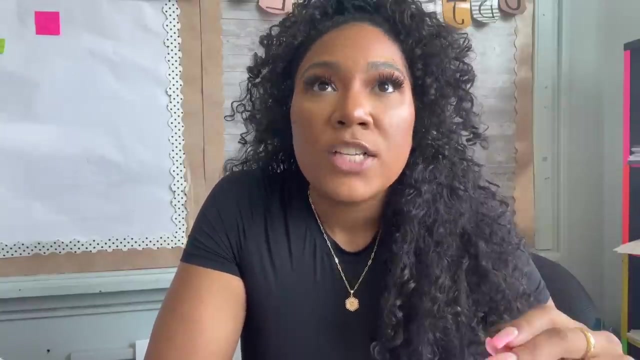 experience: teacher burnout. i've gotta be honest. i'm trying really hard not to be upset because of my computer situation. like i've been really challenging myself to post three videos a week and sometimes it just doesn't happen because my full-time job requires a lot of work, so my schedule doesn't always allow for me to get three videos up, but i'm 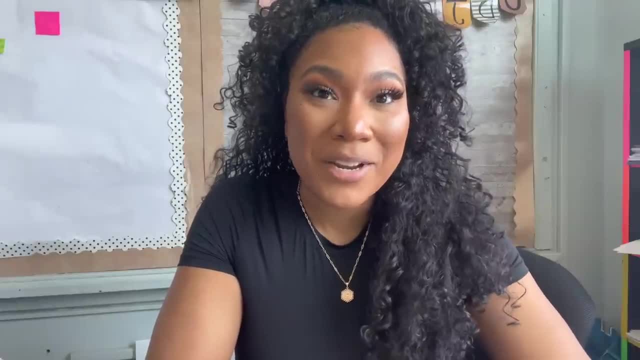 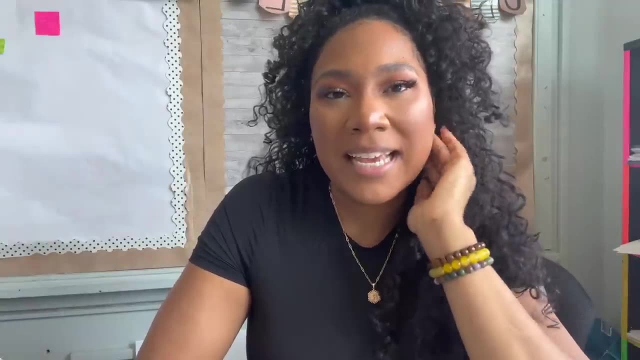 upset because i really was grinding this week to get this third video up and, like the whole thing was edited, i finished it. i should have just exported it and put it in the queue. i 'm more disappointed than anything because i've just been really challenging myself to do it and 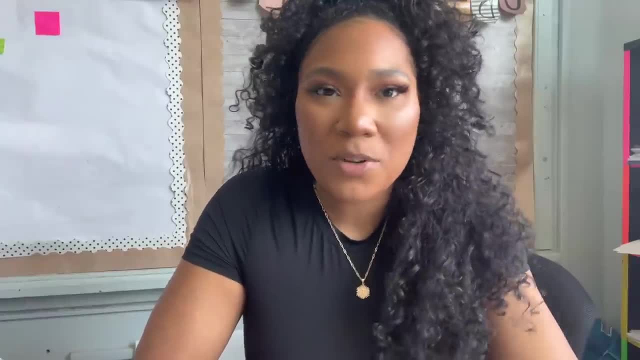 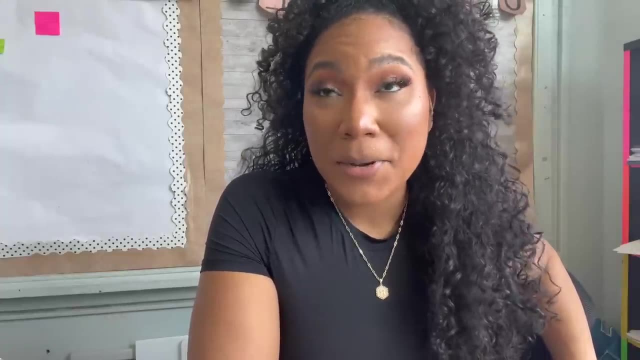 i was like: wow, this is gonna be the time that i get it done, so hopefully you guys show me some grace there, because this was really out of my control. i know with every setback there is a comeback and god is still good regardless, so it definitely could have been worse. i think i'm gonna. 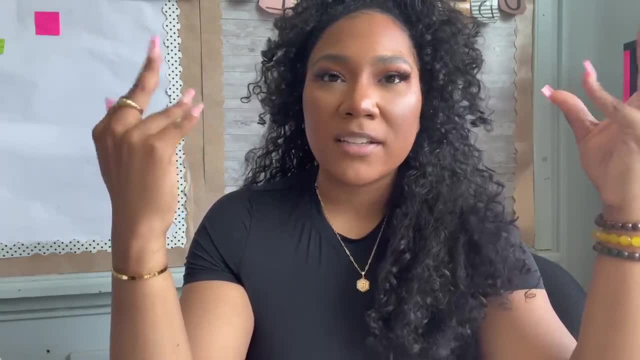 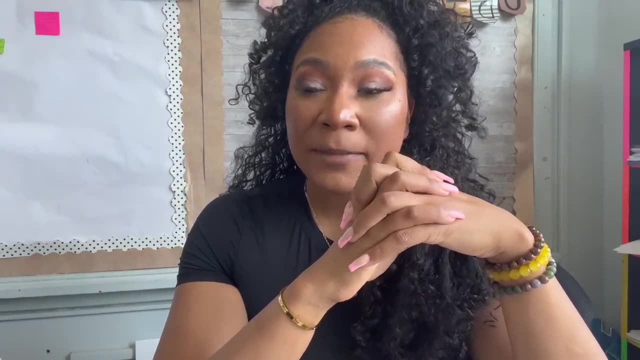 do my devotional. maybe i'll do a devotional right now because i always feel better when i talk to god or just pray or do something, because i need to like clear my mind so that i'm ready for my kids when they come in for caring school community at the end of the day. hopefully that makes me feel. 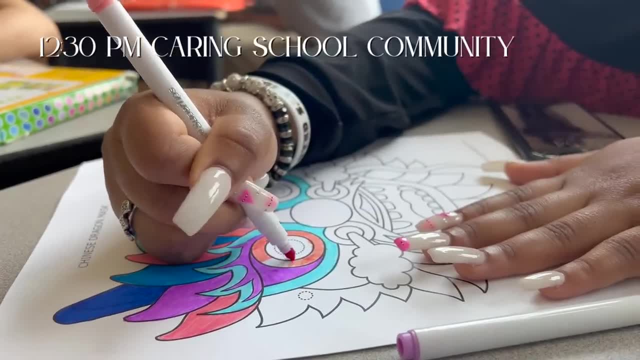 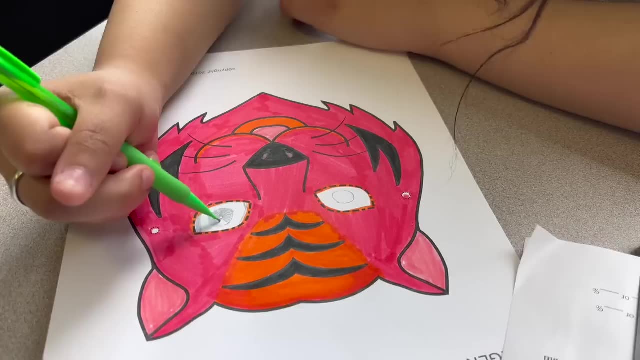 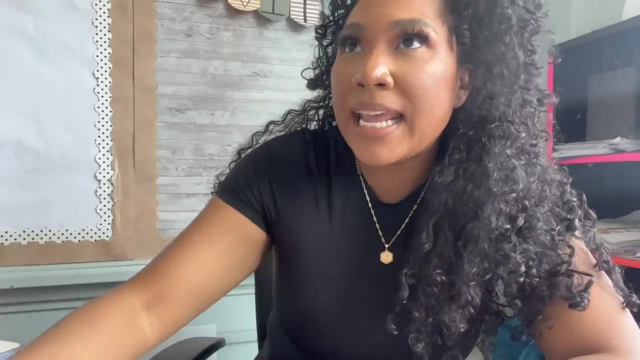 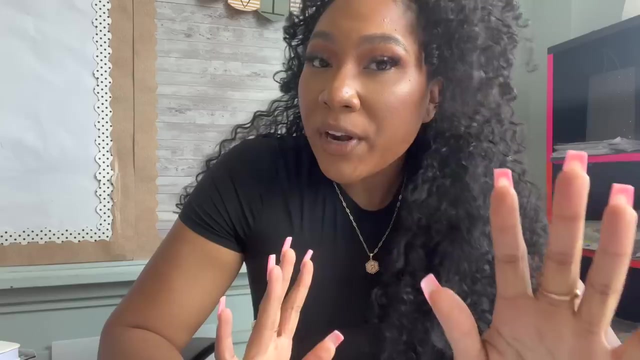 better eventually whenever i figure out what i'm doing. okay, so my kids have now finally been dismissed and it's about 1: 20 right now, so i'm getting ready to prepare for our professional development. so 1: 30, i'm gonna head downstairs to the library and 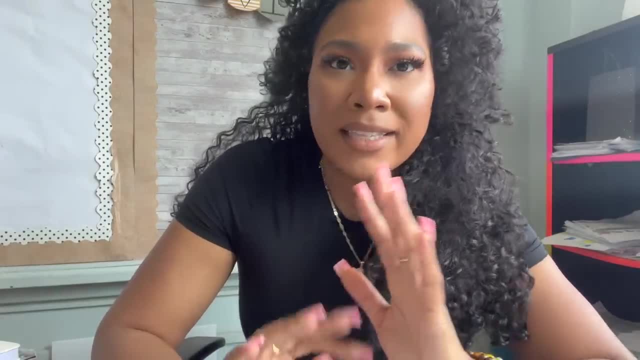 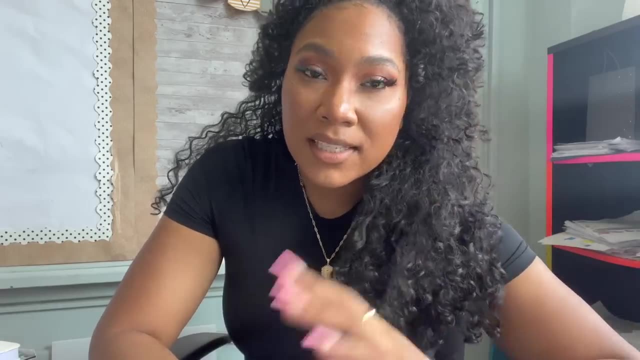 go for the eighth grade end of year meeting and then it deals with graduation and like the rest of the field trips and stuff that we have for the rest of the year, incentives, things like that. and then i have my math plc from, i think like 2 to 3, 30 and 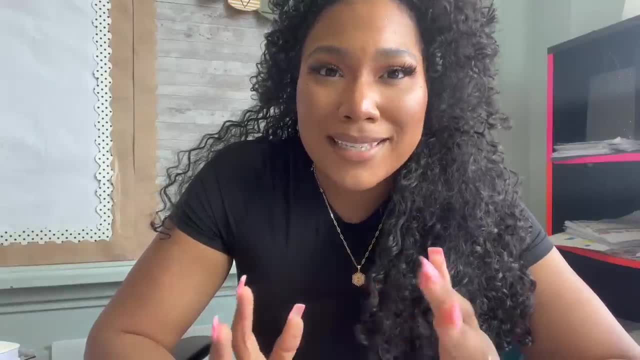 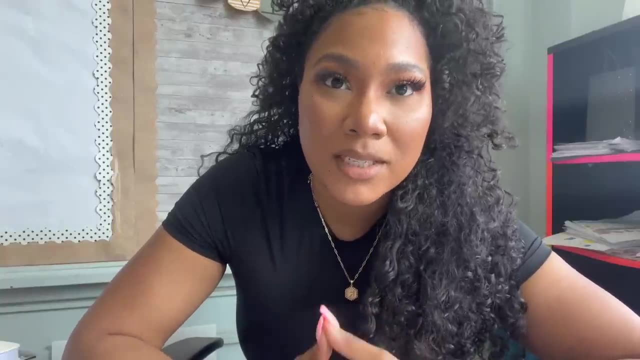 then i'm done for the day, so i'll try to put some footage in there so you guys can kind of see. but it's rather boring, it's nothing really exciting. it's a nice little break because now i don't have to talk. the pressure's not on me to really talk, people can talk at me. i'm gonna go ahead and head. 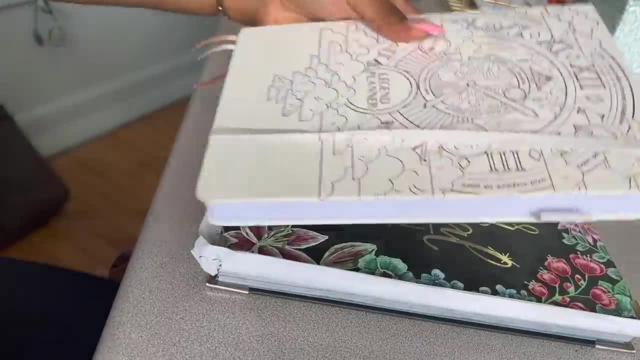 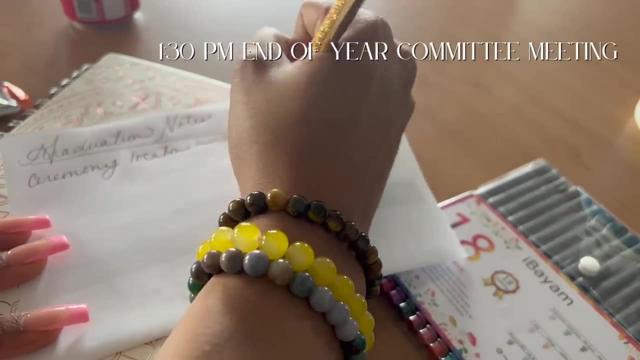 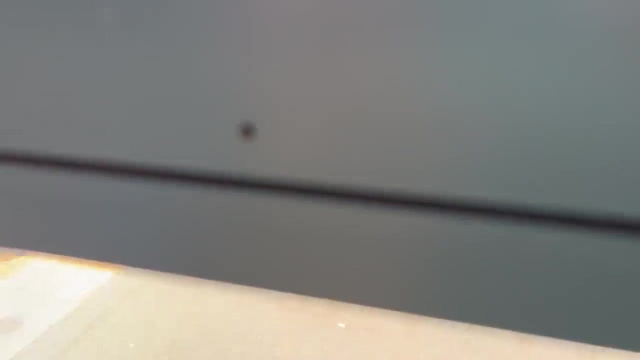 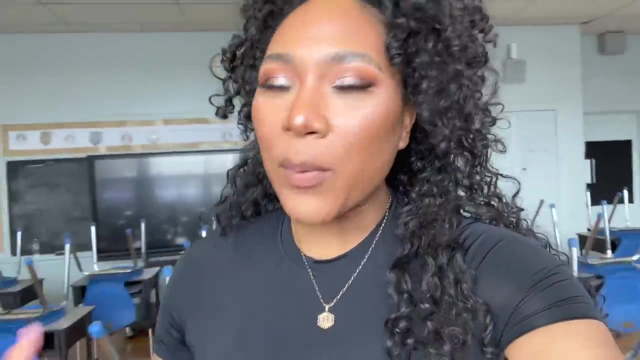 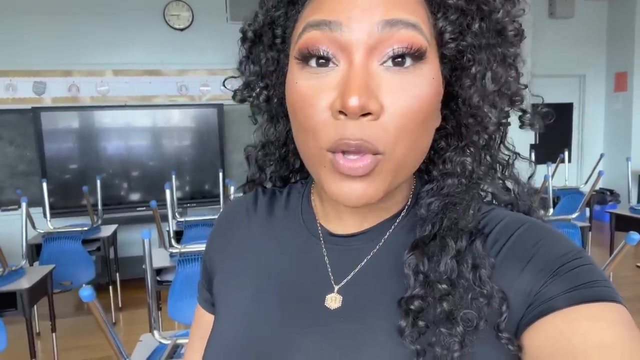 down there and then i'll check in with you guys soon. hey, i used to take myself out on dates, okay guys, so i just had an hour's worth of pd. it wasn't worthy of filming, so basically that's all i was doing. i couldn't really do anything anyway, because i don't have a computer, but it is raining. 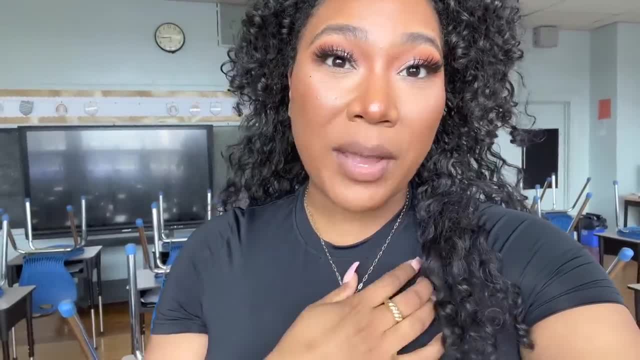 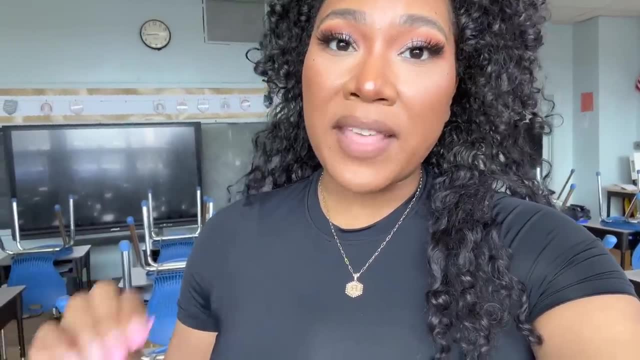 it is pouring and i need to drive to go to the library and i'm gonna head downstairs to the library and go get a macbook because i've decided i'm just going to go buy one just so i can have one for myself, and then hopefully, my school will replace the one that you know fried itself. 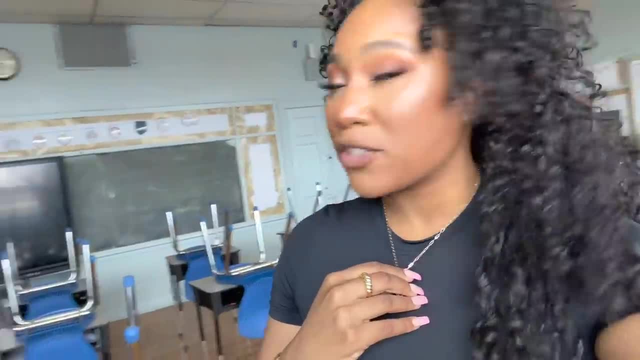 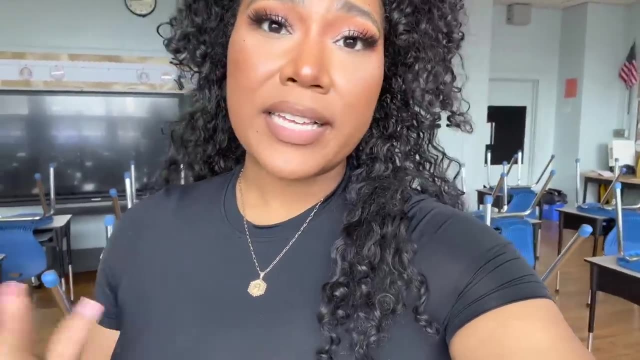 uh today. so i'm getting ready to leave my classroom, but this is what my classroom looks like right now. i have my students put up the chairs before they leave one because it makes it easier for the janitors to come in and you know sweep and mop, you know when it's their time to come in to clean. 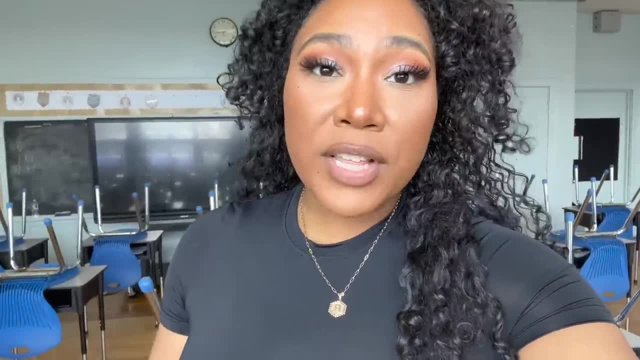 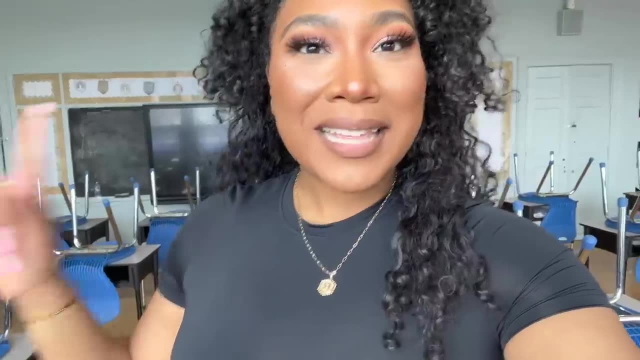 but also, um, it just puts a little bit more responsibility on the kids, making sure that things are completely off the desk, everything is put away, and then they can put the chair up on the desk because it won't be covering anything. we just got the email that we can leave, so i'm literally heading to my car. there's a tornado. 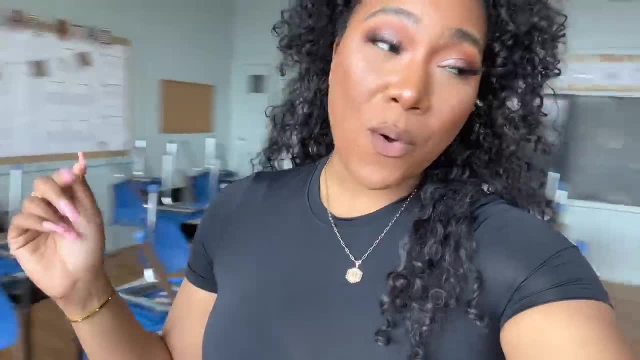 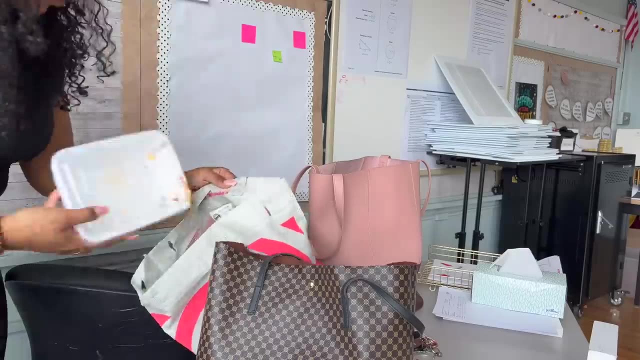 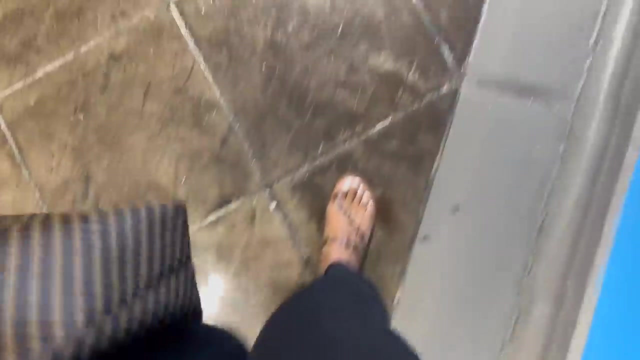 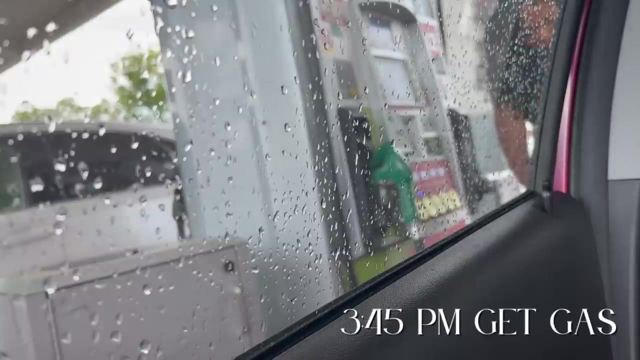 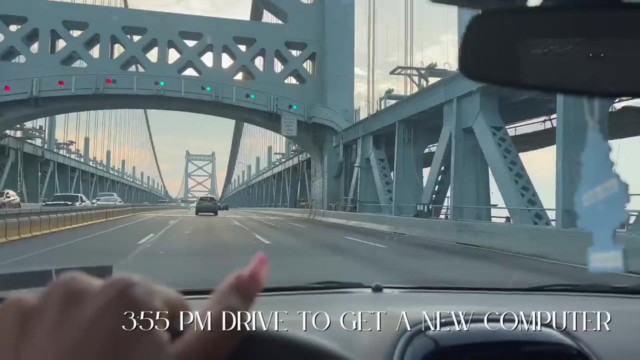 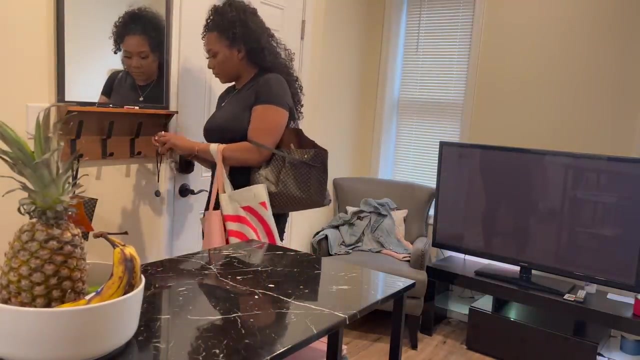 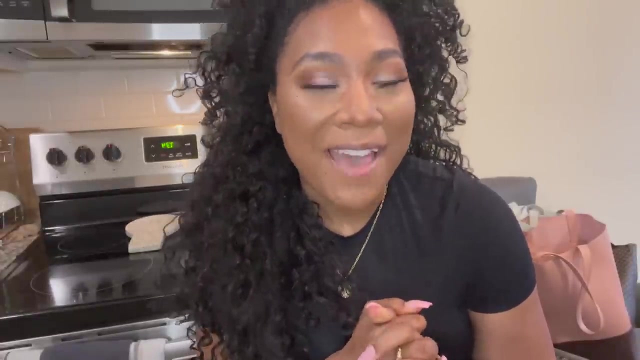 watch. so god, just cover me. i'm literally gonna be running out of this building, so i will talk to you guys soon. all right, so i just got home and i am not having the best day. this whole computer situation is blowing me. the laptop that i needed or want to use is not working, so i'm just gonna go home and 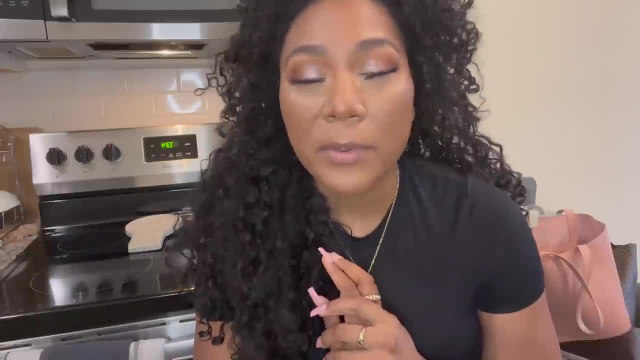 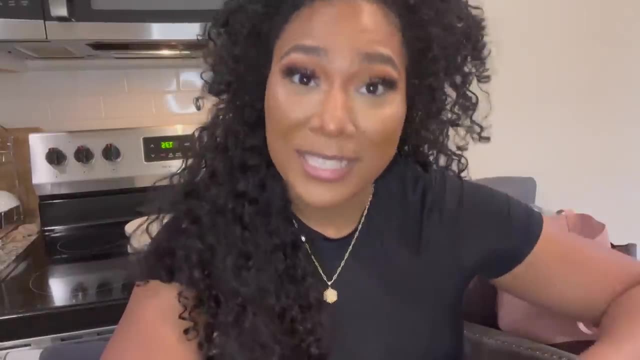 make sure that my laptop is here also, because i don't have a laptop. so i think my laptop is gonna be able to survive this whole time because i think it's gonna be home soon. so, first of all, i just got home and it's sold out everywhere here in philly, so right now i 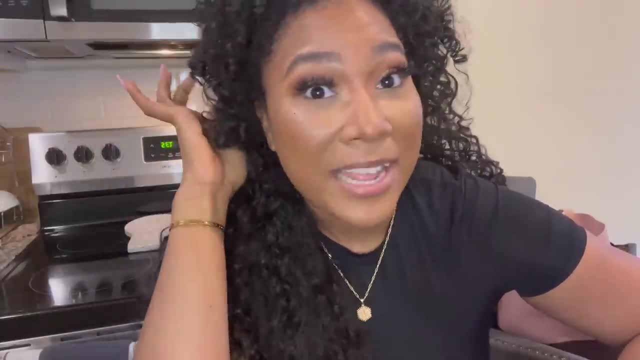 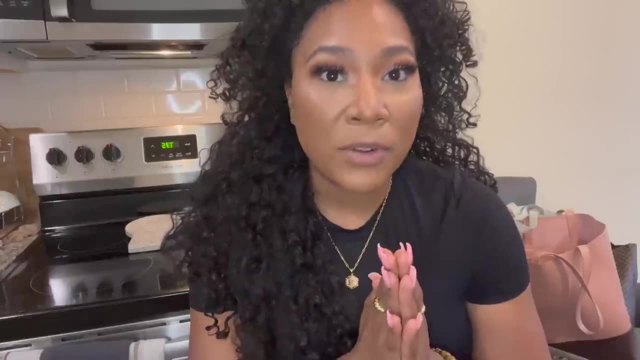 am just got home, i'm gonna change it to some comfy clothes, because your girl has been in real people clothes all day. i ordered some takeout because i'm treating myself, because i just not having the best day. i ordered a poke bowl, so i think i'm gonna go change, wait for my food to get here and then i'm. 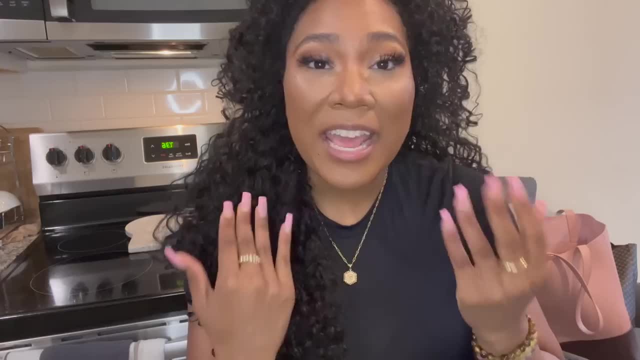 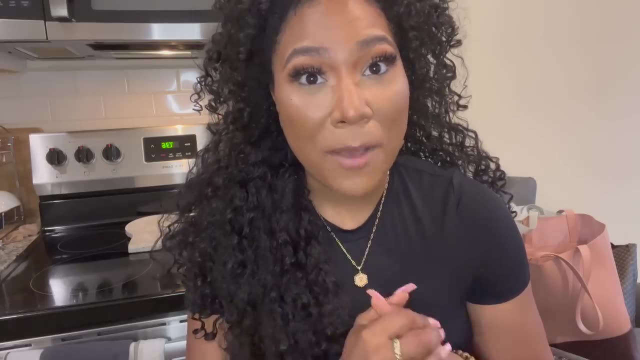 probably going to like do my devotional. i didn't read my bible today, so i'm going to do that, and i think it would just be a really nice way to end the night. in a perfect world, i would be answering YouTube comments and also editing YouTube videos, but now that I'm without a laptop right now, so 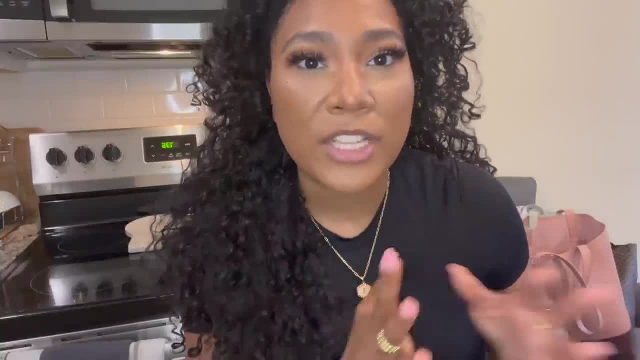 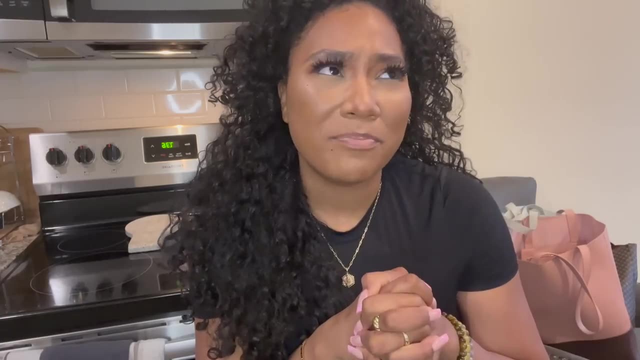 you're kind of gonna miss that aspect of my day, but just know that I would be doing that, so I'm just going to get comfortable, lounge a little bit, probably take my makeup off soon, because the lashes they gotta go. that's really gonna sum up most of my day, because now I'm just gonna be. 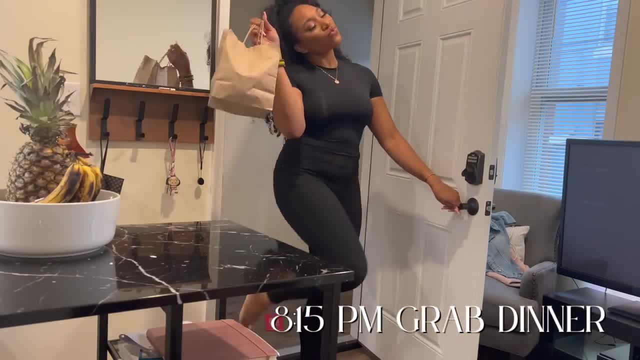 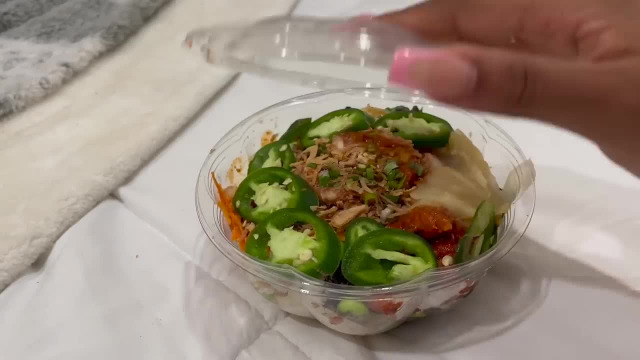 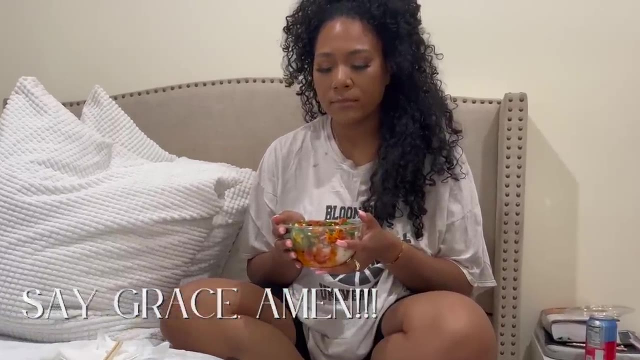 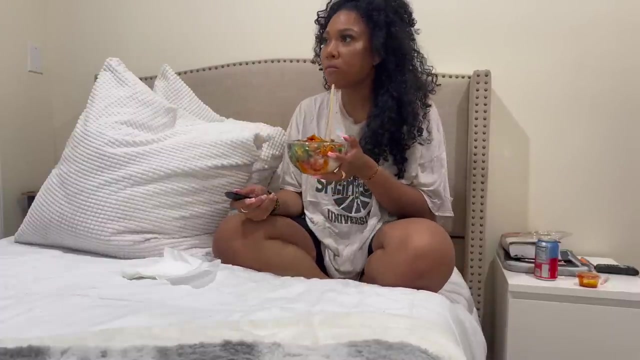 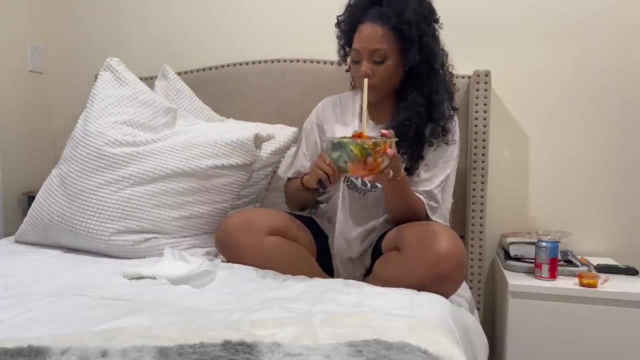 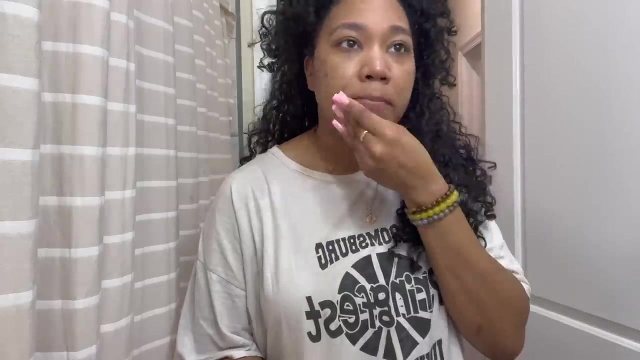 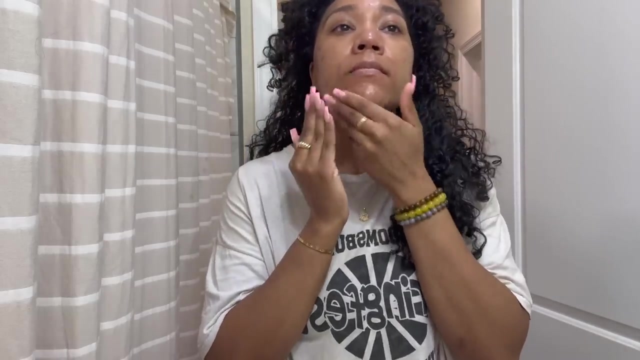 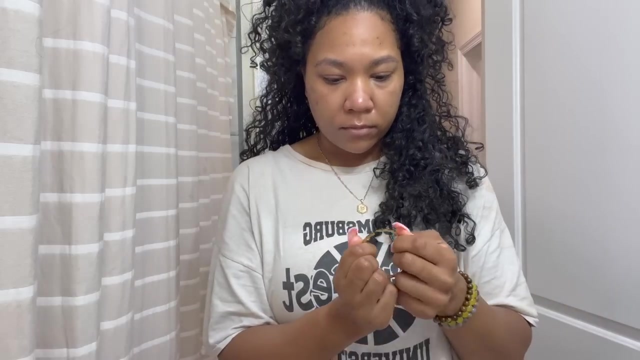 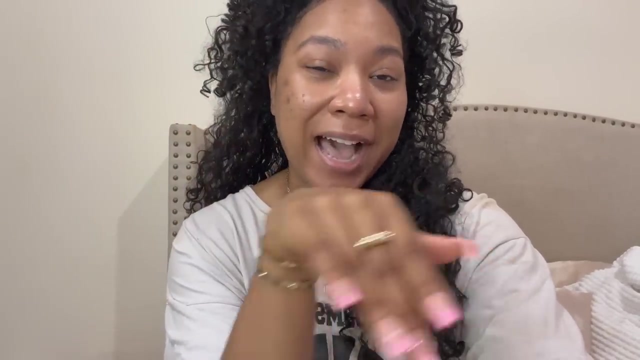 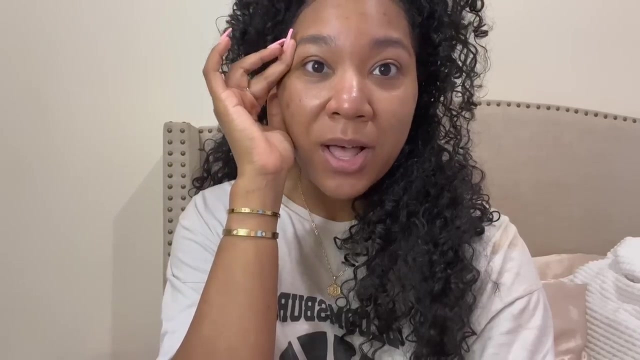 in the house. so yeah, the goods are secured. so okay, guys. so i'm getting ready to go to bed. i'm so tired. i watched an entire service from the transformation church series- i think it's called cuffed- so i watched the very first episode. it was two hours long, so i had my dinner, i watched that and then i didn't end up doing my 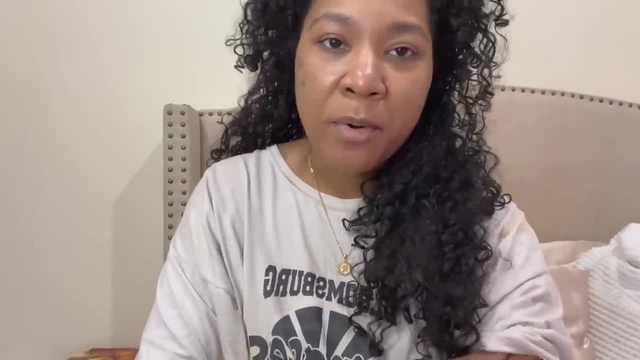 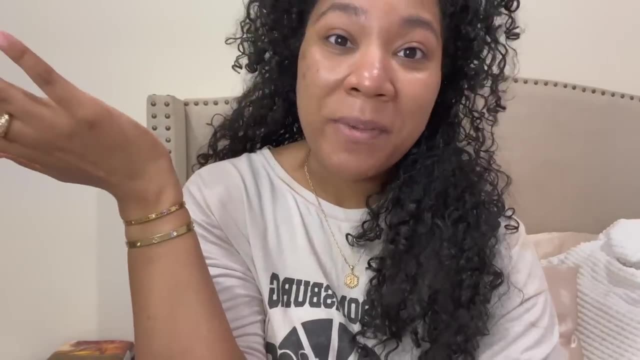 devotional. i just, you know, was paying attention to the sermon and then tomorrow morning when i wake up i'll just make sure that i get my devotional in first thing. but that's basically going to conclude a full day in the life of a middle school math teacher. it's not that exciting. 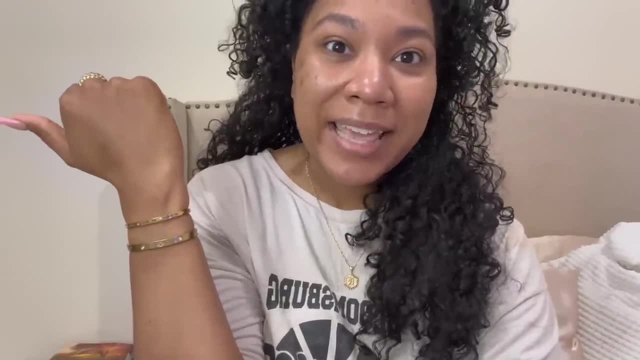 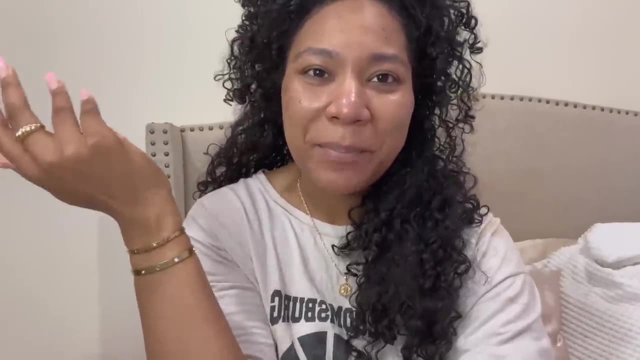 but it's very realistic. nine times out of ten my days look like this: on the off chance that i go out after work. it's very, very slim. sometimes i do, and maybe on a day that i do that i'll film, i'll update it, but i definitely think that it's so beneficial. 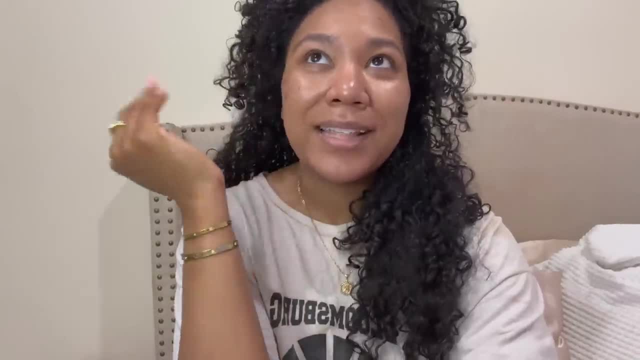 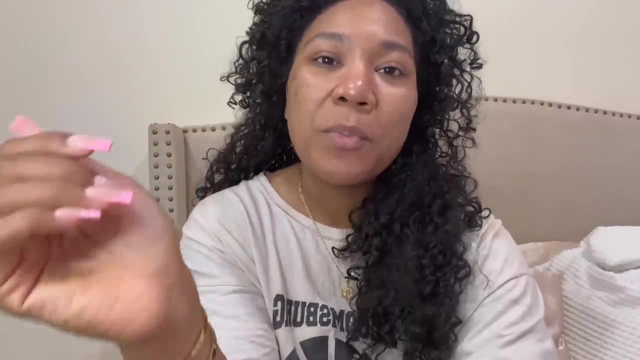 to show the reality of what teachers go through because, like, the job really doesn't stop. thankfully, tonight i didn't have to do any emails, i didn't have to do any grading, because on the weekends i think it's so important that we give ourselves a break, like, don't take the work home. 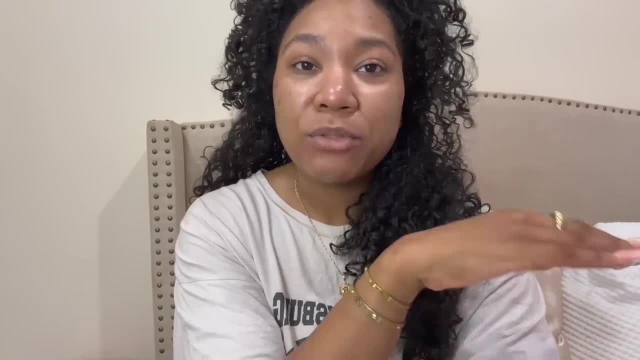 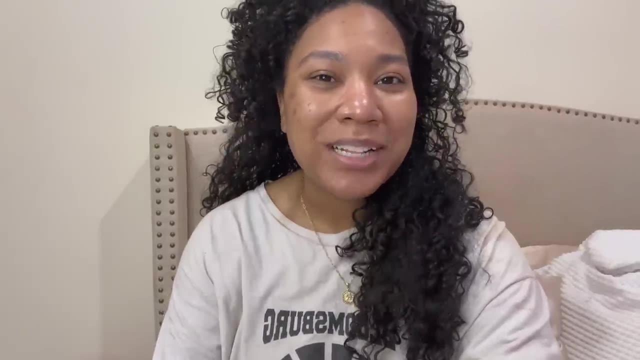 with you. you work five days out of the week for 24 hours a day. like you don't stop being a teacher. like you're bringing work home, you're coming to school early. give yourself a break on the weekends. if you enjoyed this video, please be sure to like, comment, subscribe and share. also be sure to turn. 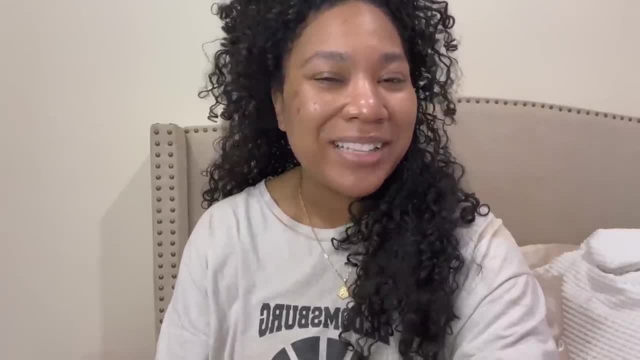 on your post notifications. that way you can be notified every time your girl drops a new video. and until next time, babes, i'll see you in my next.